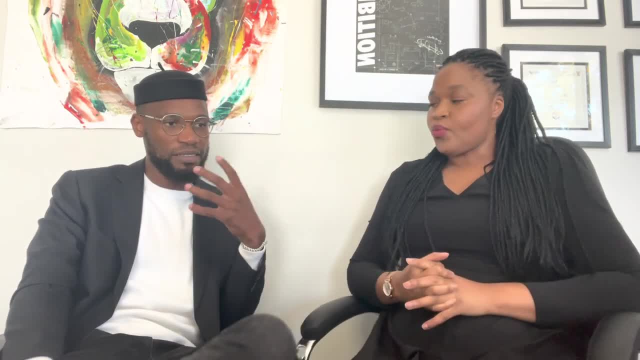 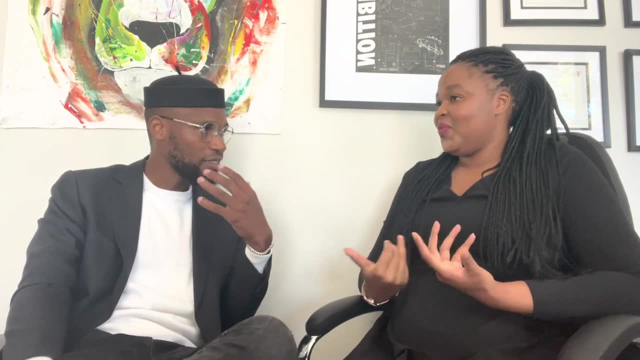 And the reason why was now I was aware my brother was already finishing his accounting. he's an accountant, He was already finishing his accounting degree, so he was already giving me insights about what is happening in tax and I was already inspired. 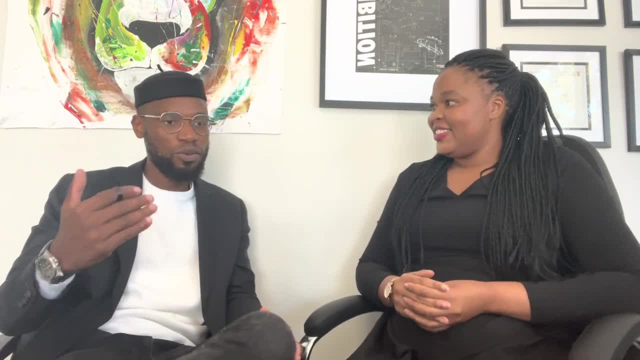 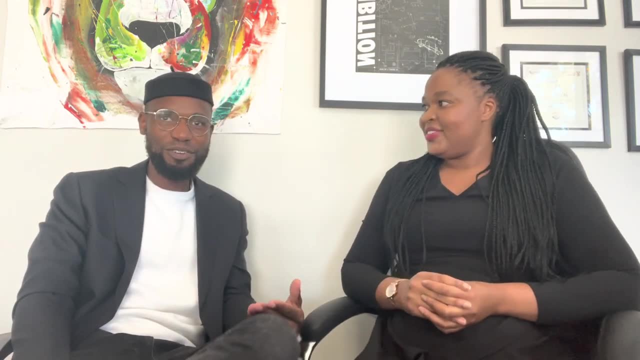 So because of that I was. I aspired to study econometrics or statistics. So when I get there, I think I applied and then I was. I think I was rejected for econometrics Because of my marks there. Oh, okay. 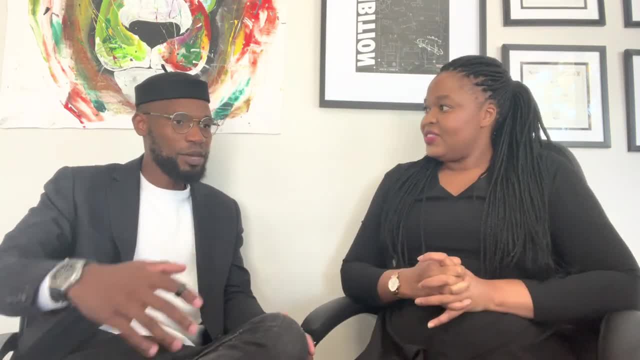 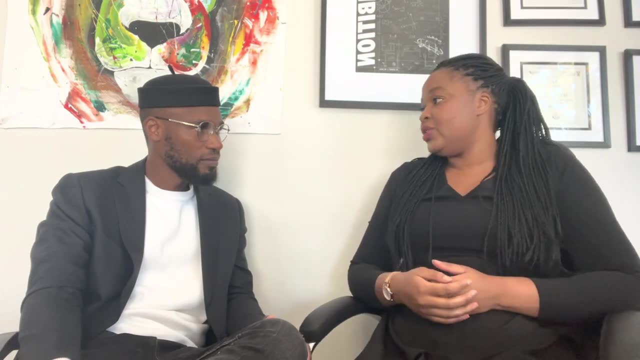 But when I got there, then I finally applied for statistics and then I majored in econometrics. Oh, that's so cool. That's so cool. And normally people that get into stats- Math stats- are people that want to get into actuarial science. 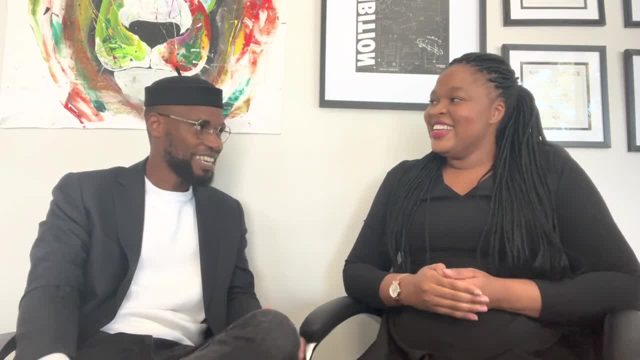 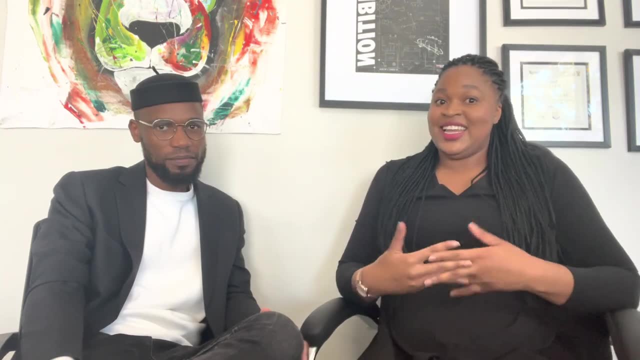 Yes, yes, I also had interest in that, but my marks were not going to get you. They were not going to get you, but it's okay. And then so tell me, how were you? were you an outgoing student or you were just a nerd? 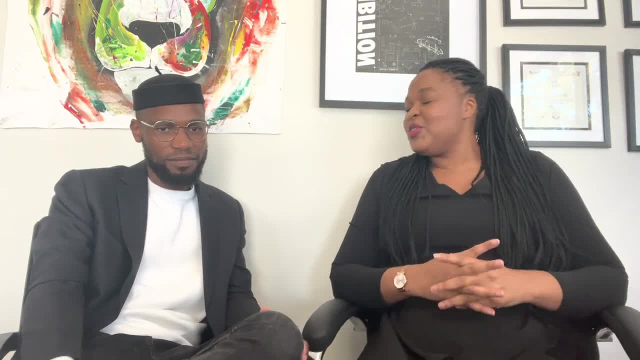 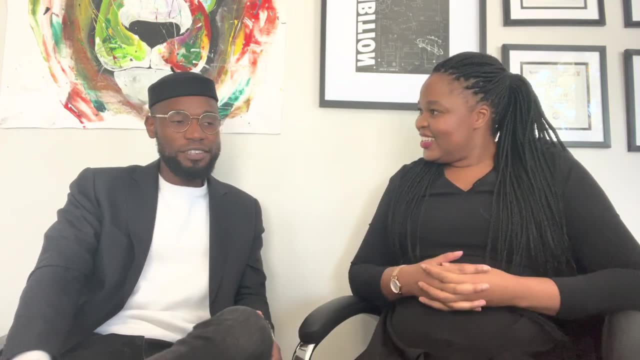 chilling at home, always studying or always going, you know tax. back then had that. you know square side of things. Yeah, yeah, yeah. So were you that person that goes to square? you know? High school- I was outgoing because I think I was already outside them. 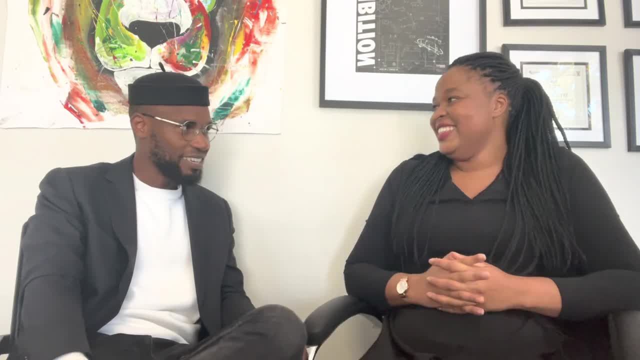 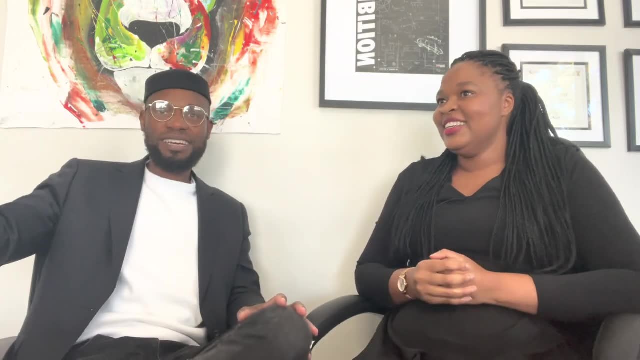 I was already advanced, Okay, When I got to tax I was just failing, So because of it, it turned me to an inside person. Oh, Luke, our auditor, he's also. he was with me. I remember he used to come to my room rest when we were staying in Holyrood. 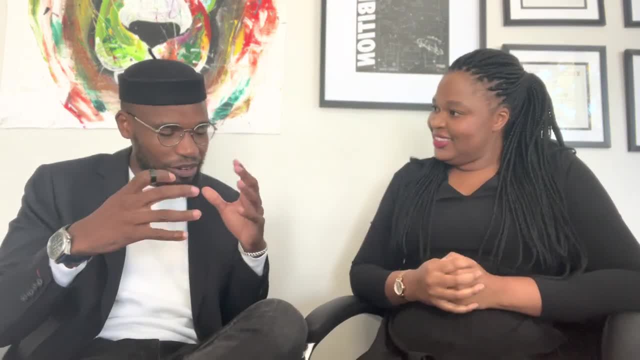 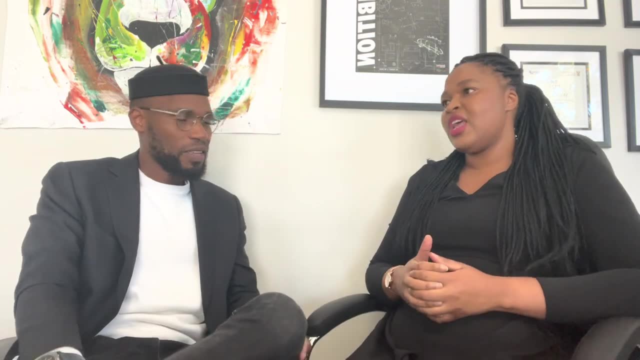 Yeah, I became an inside person just studying. It was because I wanted to figure it out, But I'm not really an inside person, but tax made me start to think like that And that's actually a good thing, you know, And the fact that you're just here, you know. 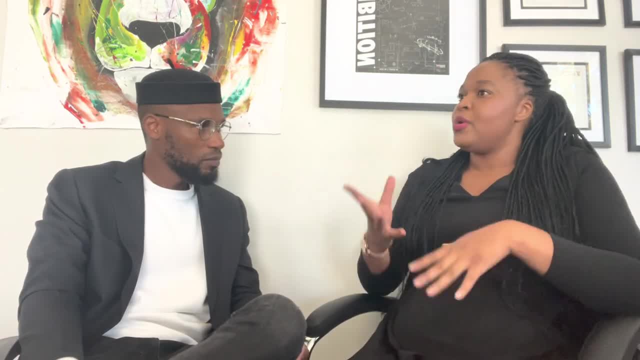 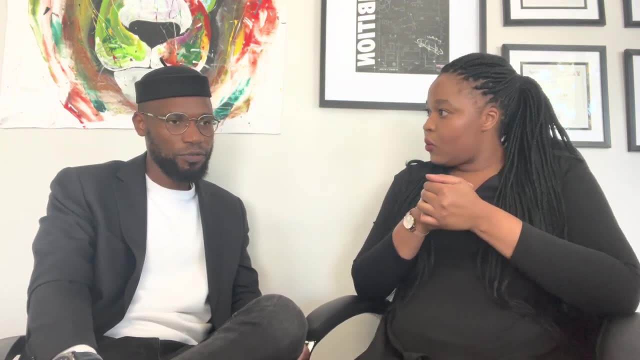 So I wanted us to have like the things coming from it's from uni, and then after you went to you went to the corporate. I went to Marsmart. Yeah, I consulted for a company. So after university, tax taught me a lot. 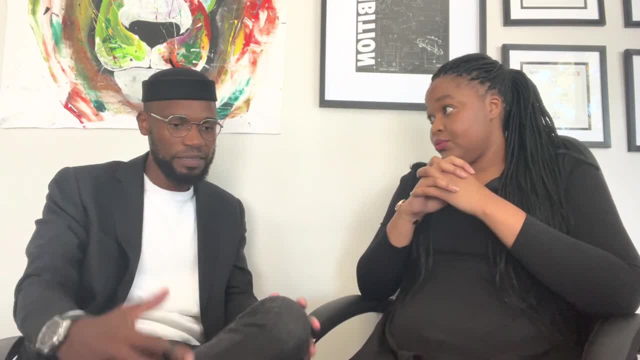 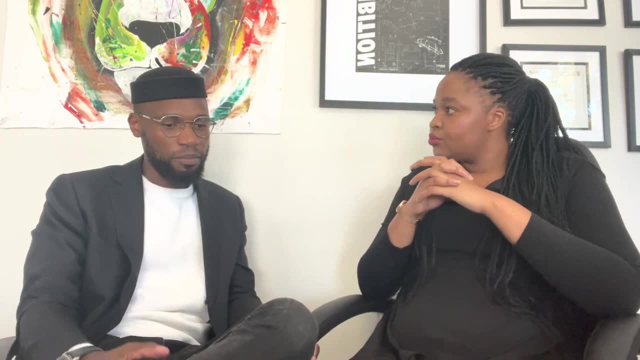 You know you fail, then you pass. you try to balance your things. Something I learned about myself at tax was: I adapt. I adapt on situations. So I learned that. and then I'm 2012, I finished 2013, I started, I'm studying, I'm consulting. 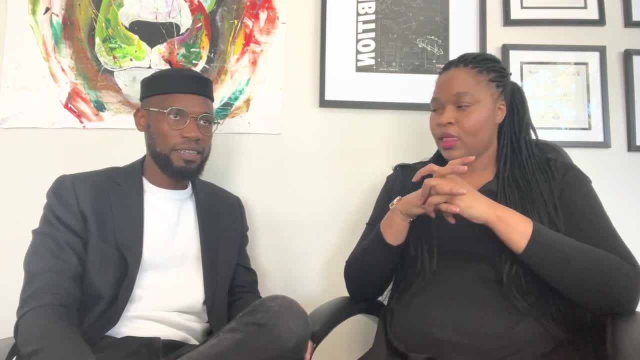 at Marsmart. Okay, I'm consulting as a data analyst, analyzing private brands. Private brands are brands that are owned by the company And I'm trying to understand the penetration of the private brands to national brands And because of that, it's a big job. 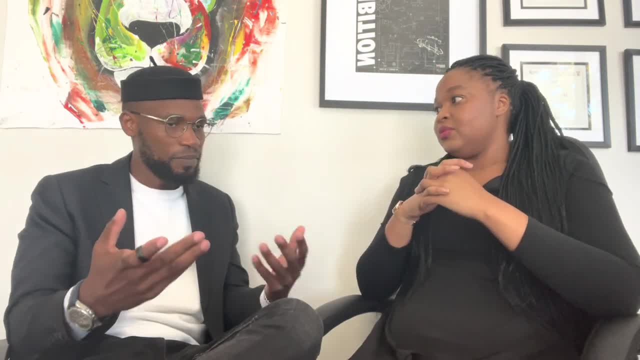 So I was, oh, I'm starting to learn things, or not? And I didn't know anything. Yeah, So I'm starting to learn things a lot. So, because I was consulting for a US company, I was like, oh, I'm going to do this. 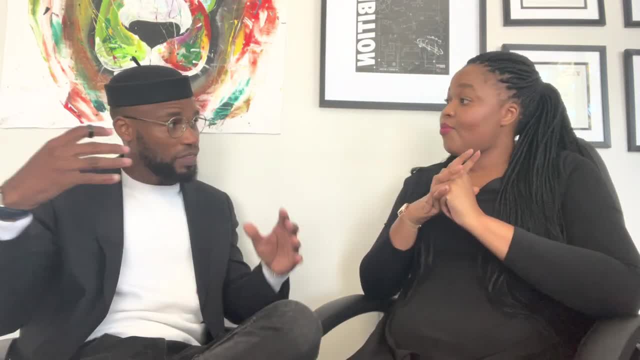 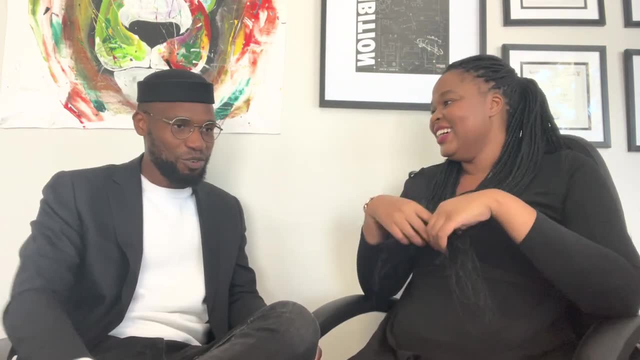 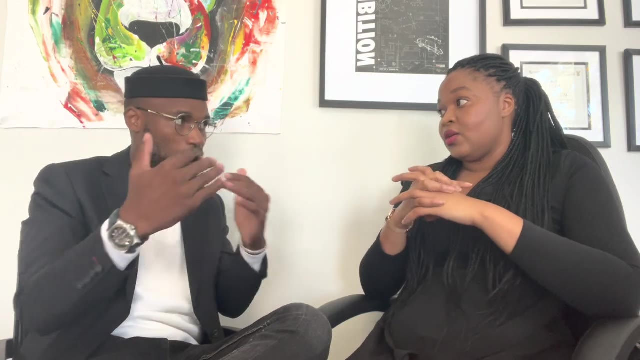 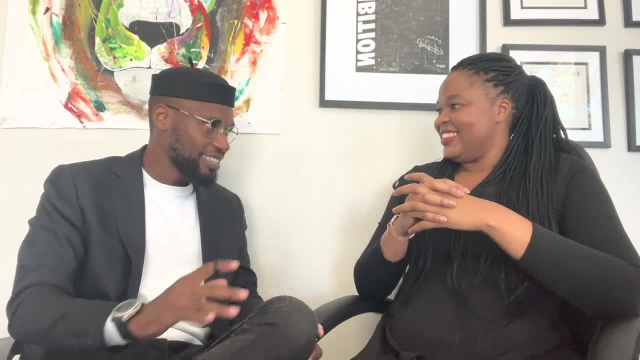 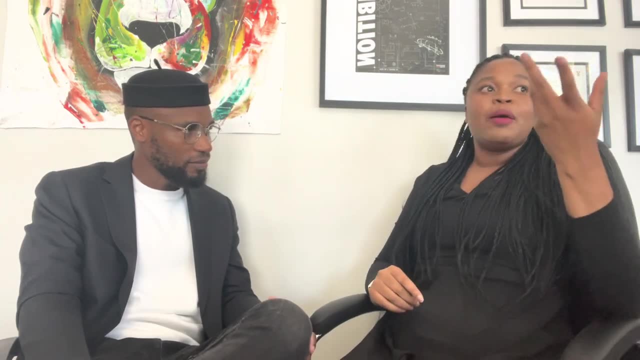 2013,. I was starting to talk analytics, Oh, okay, Okay. So I want to know, like, when did this vision come in? Because you know there's something about life where, when you're going through a path, right. 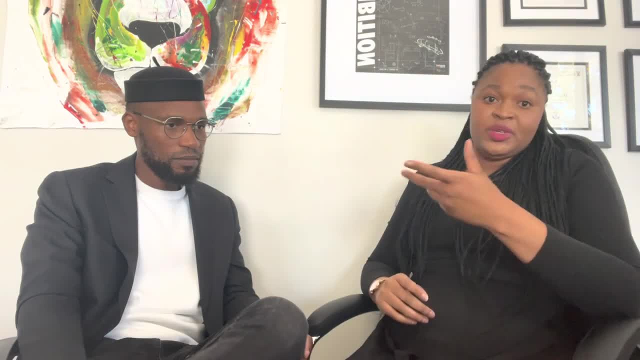 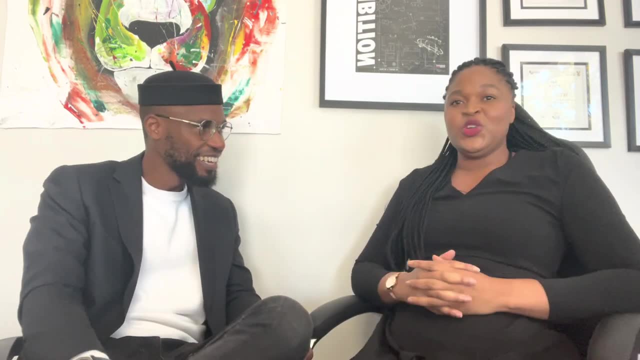 In high school you were probably thinking that you want to be a doctor- Yeah, Or you wanted to be- Yeah. you just want a money- Yeah, You just want a money. So want to go to uni. you know everyone who goes to uni is just there: happy, chilling, living their. 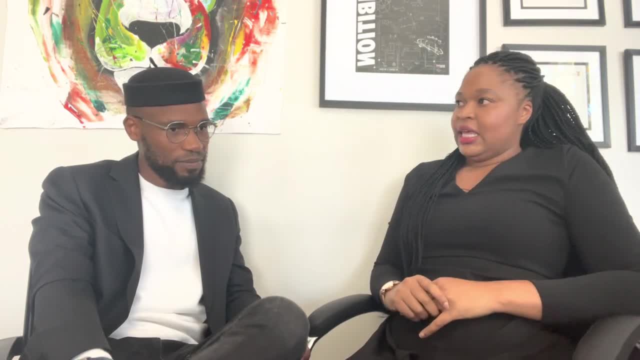 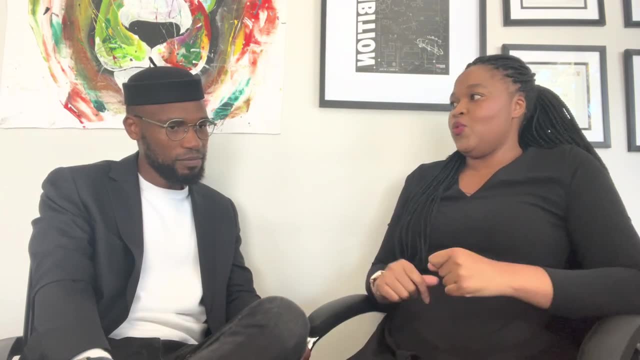 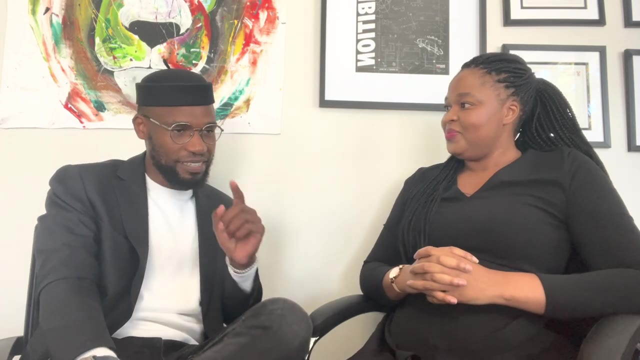 best lives, you know. and then when you get to varsity, like there's so much to do, so much you know, and then after when did this vision come in and kick in? when did that thing just click and be like, yeah, i like that question? it clicked 2013.. but 2013, i'm coming from louisville in 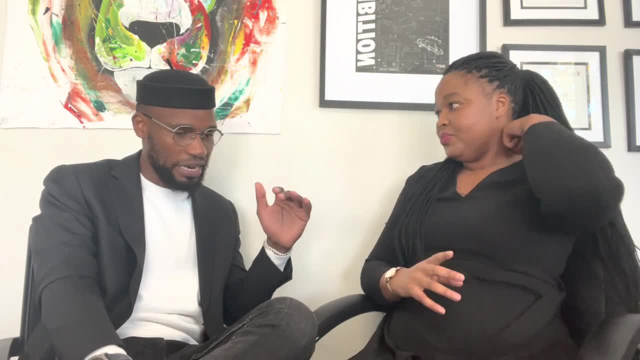 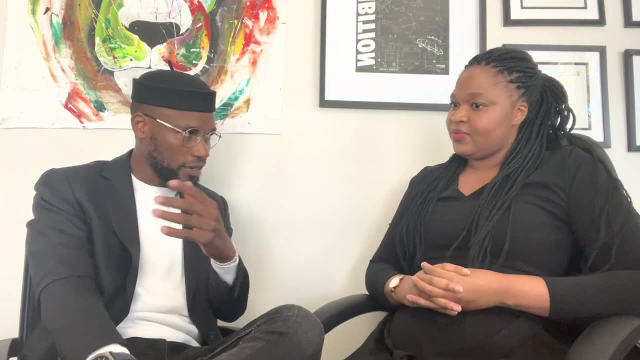 louisville when i was 10, i was selling 10, 11, 12, 13, 14, 15.. if i was not selling, i was working at a farm and i was helping them ship their veggies to spa and checkers. so my upbringing is about 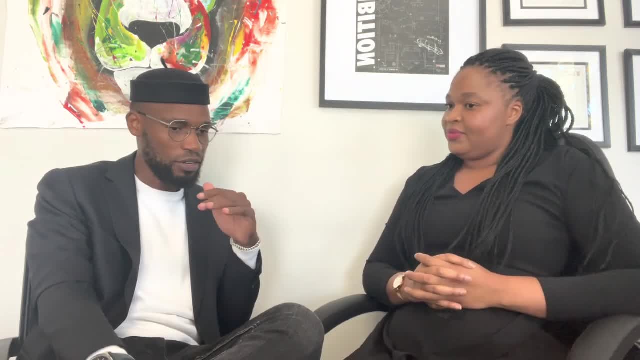 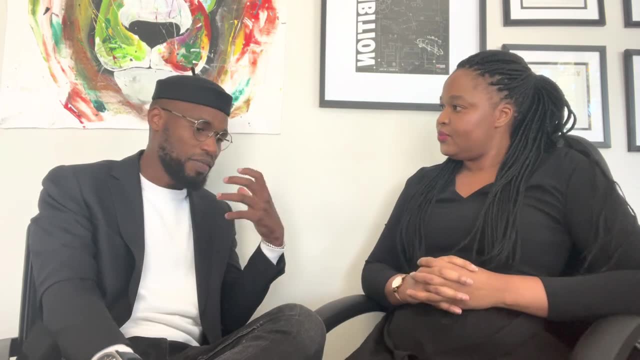 entrepreneurship- okay, okay, hardcore entrepreneurship. so i can't say i'm disadvantaged, but i'm growing up in a very diverse environment where i'm able to see what is going on. so that upbringing allowed me now, when i think of entrepreneurship in 2013, to be able to make sense of what. 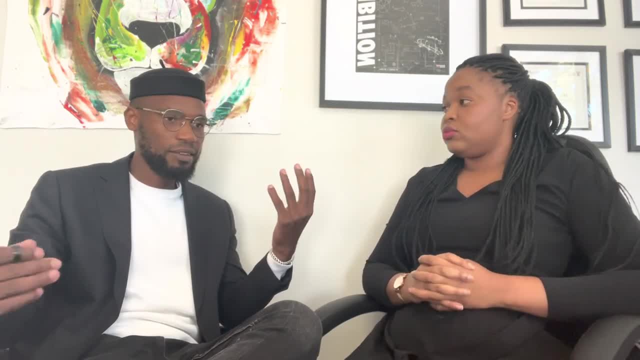 is going on and to be able to make sense of what is going on and make sense of what is happening. entrepreneurship is Because even when I was at TACS, if we're talking with guys, I would still bring business in. I would still tell them I'm going to do business in the future. 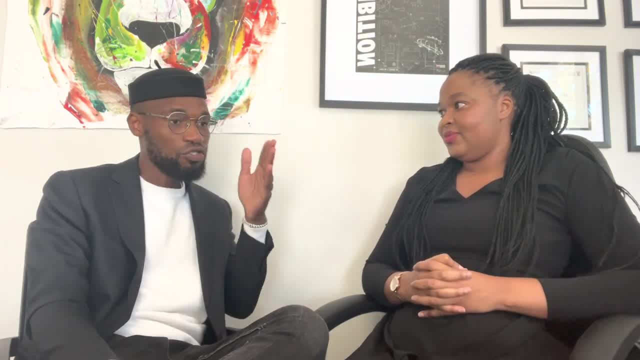 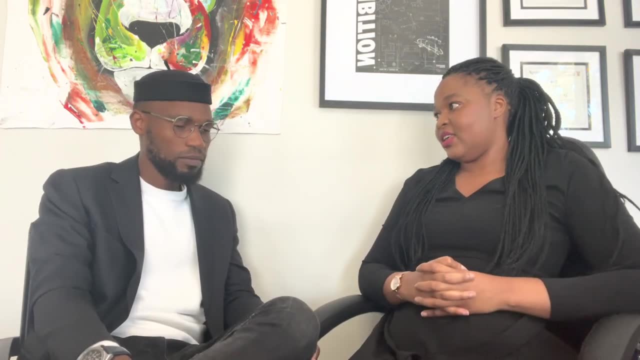 even though I didn't know what it is But 2013,. I got to know what exactly I'm going to do through that analytics, So you knew at that time that I want to start my thing, and then you worked towards it. 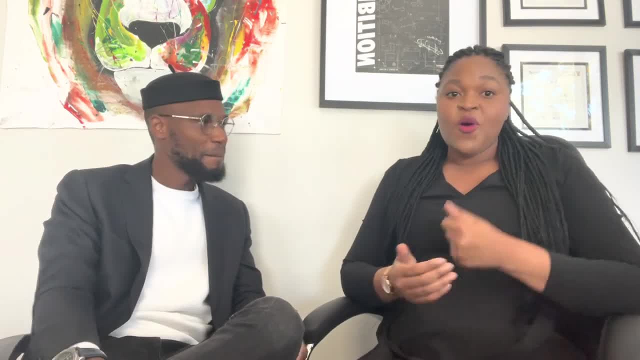 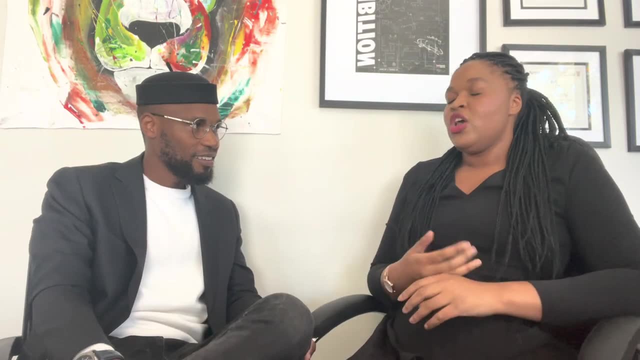 My first year. Look at you right now, because I won't lie: in Africa, tech is still on its primitives, Like we are still on our primitives. You can literally see there are so many corporates that are also not. They are not doing it. 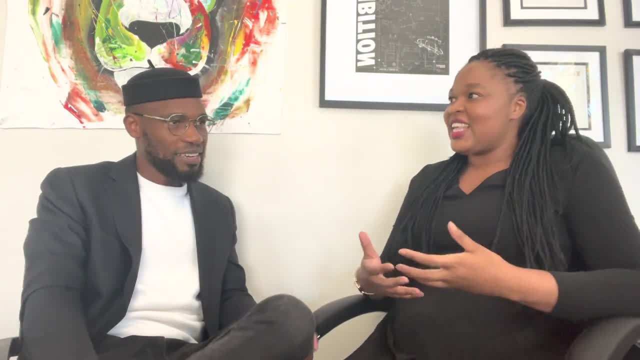 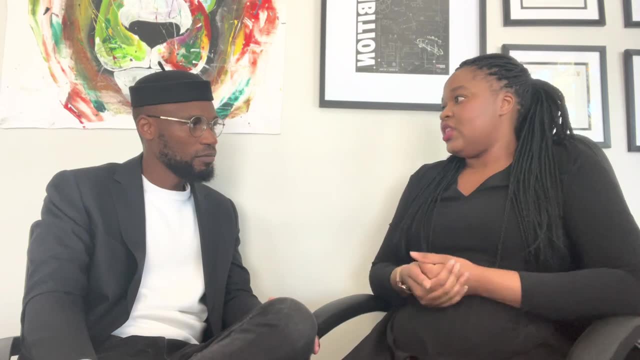 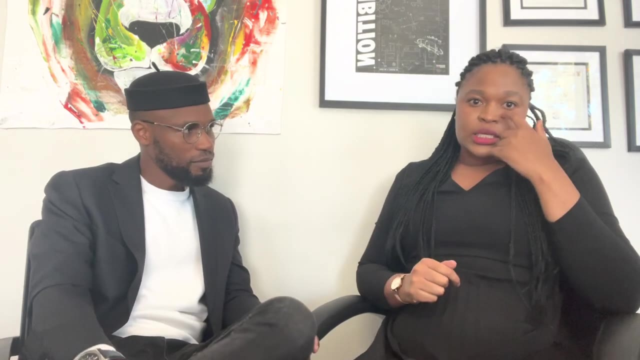 They are not doing it, They just do a part of it. They do a part of it. And you, We thought leading Yes, And you literally just were like I'm going for this. So obviously, when you went for this, it was really hard. You had hurdles right, Because, to be honest, I'm one of the 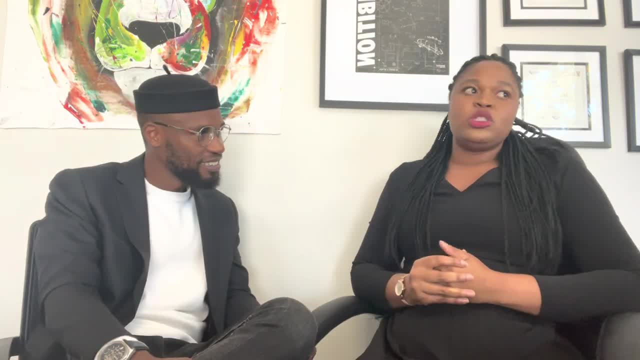 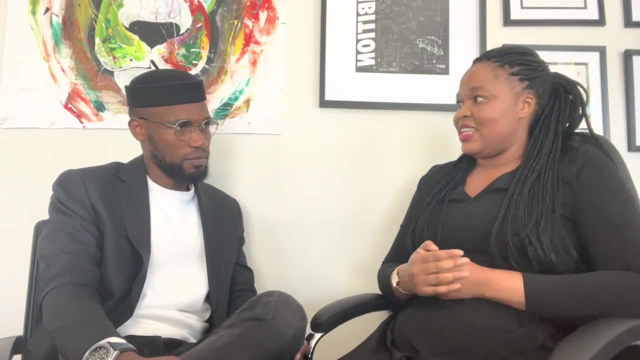 I don't know. I'll tell you, I'm one of those people That you know how, when people get into entrepreneurship, they now start bashing 95ers and they're like: why are you guys? I have my own time. 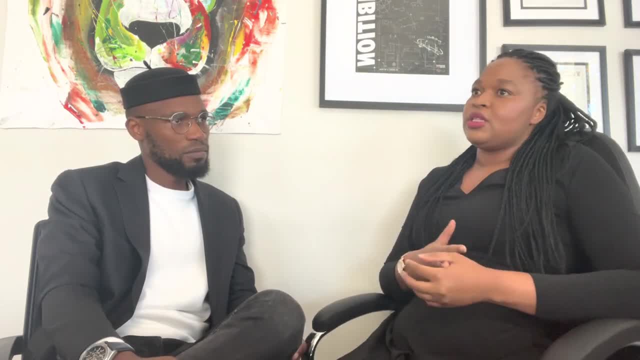 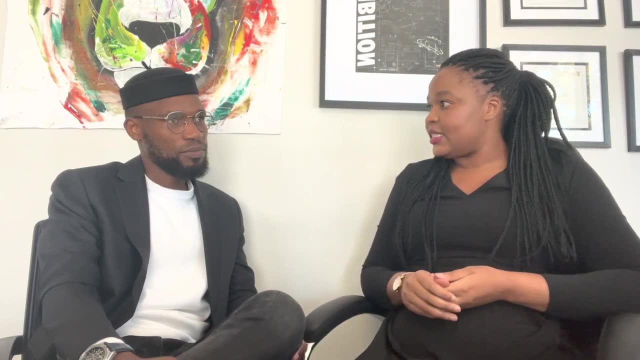 I can do this, I can do that, And I'm like sometimes there are people that we all need to start somewhere, And I think that was the combination is wrong. Yes, It shouldn't be like that. You know why? Because even when you're doing this entrepreneurship thing, you're not alone. 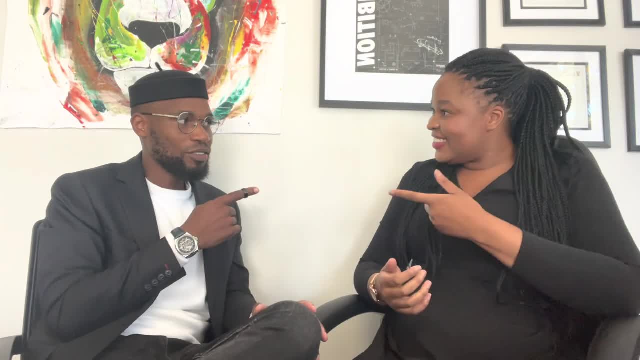 You have to build a team, A person who says that is still alive, Check them, Check them, Check them properly. They're not unemployed anymore Because it's about community, It's about working together, And once you start working with people, you respect people. 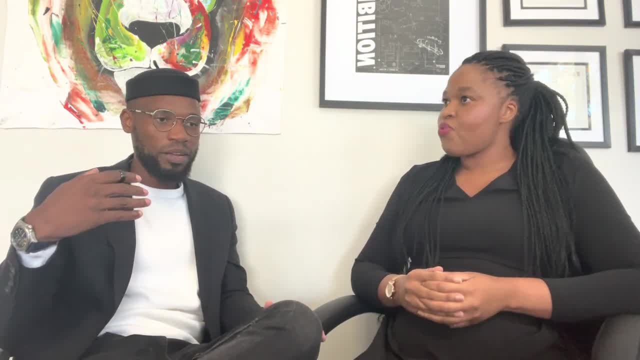 And you start realizing that our growth, my growth, is dependent on them growing. So we all need to grow. It's not about. it's not a one man show, So I don't speak that because it doesn't talk. I can't speak like that. 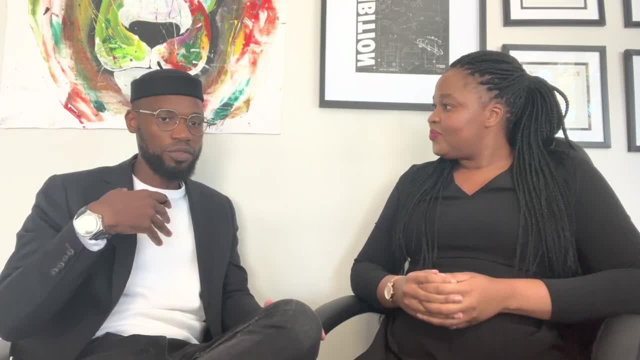 I've got so many professionals. Look at these guys. They are more creative than me. So what am I saying? Yes, So I don't speak that because it doesn't talk. I can't speak like that. I've got so many professionals. 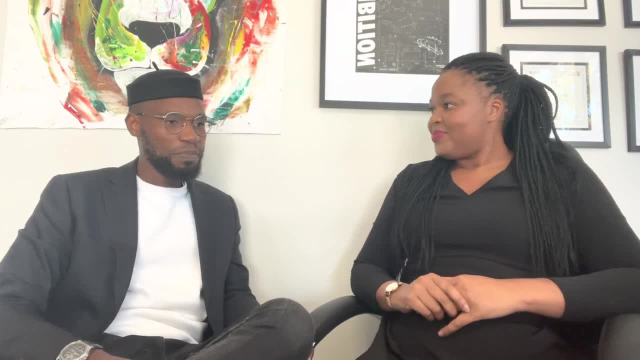 Look at these guys. They are more creative than me, Exactly. So what am I saying? Yes, Guys, you heard it from him. Yeah, Literally, you heard it from him, And I like your view, because I've always also viewed it in the sense of how can you? 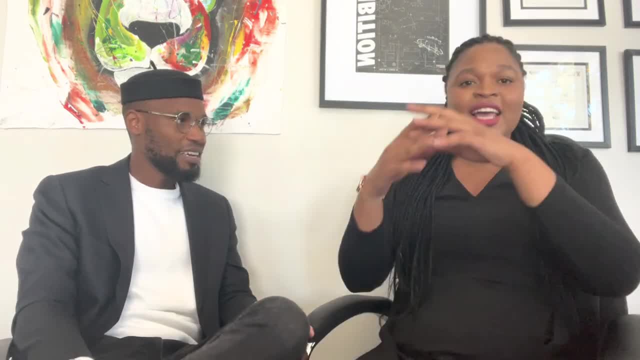 say that, while we know that you need someone, Like you need to employ people, You can't really do that. Which corporate does a person have? It is so huge and they are not. Yeah, Nothing, You know. Yeah, I don't speak that because it doesn't talk. 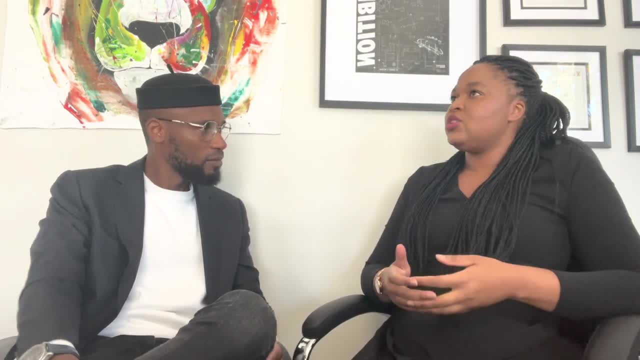 I can't speak like that. I've got so many professionals. Look at these guys. They are more creative than me, Exactly. So what am I saying? Yes, Guys, you heard it from him. Yeah, Literally, you heard it from him. 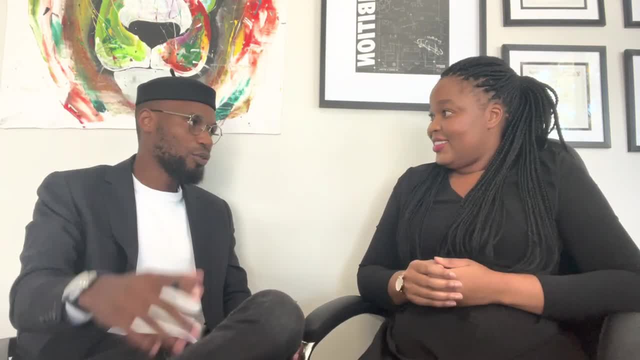 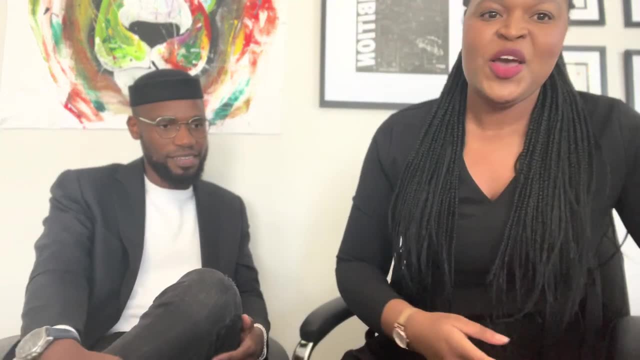 You can't really do that. Which corporate does a person have? It is so huge and they are not. Yeah, No, Nothing You know. Yeah, I'm so happy I have made a few questions, right? Yes, Yes, 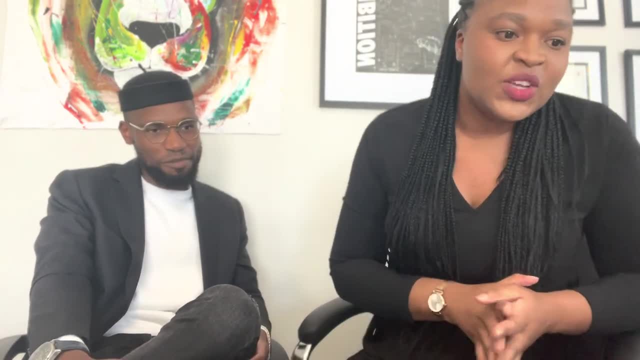 Because you know guys Like I can talk for the whole day. Yeah, So yeah, Just to have a young talk back. Yeah, If you had an interest song played any time you walked in a room, what would it be If I had an interest? 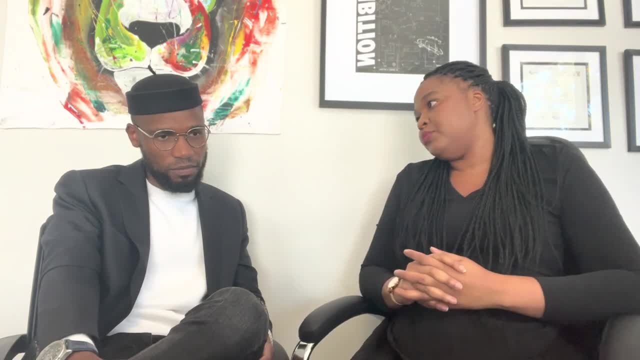 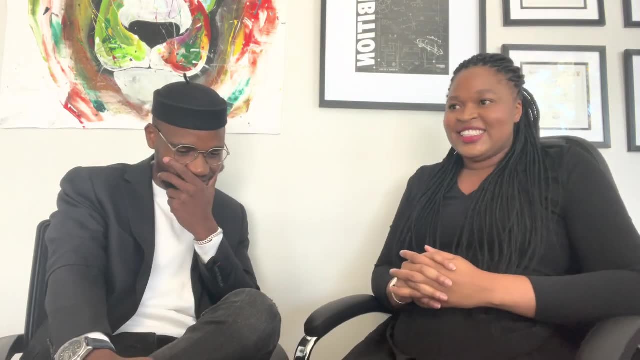 Intro song, Introduction song. Ah, That Very When you Girl Girl Girl, Girl, Girl Girl Girl, You know what it is. You went inside the room and you just like, I want them No. 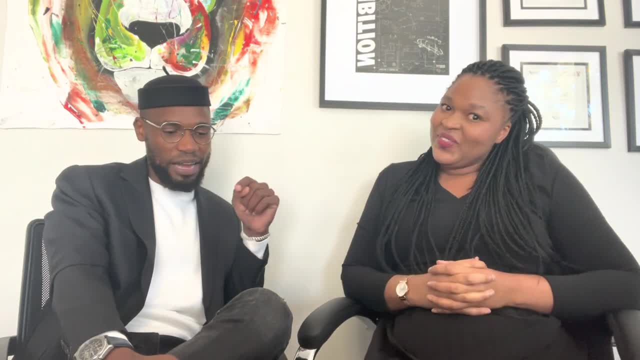 Let me give a shout out to. I'm just gonna. I was gonna go in with Jay-Z. They told me I was going to go in with Jay-Z And a movie with a song called You Don't Know. Oh, Okay. 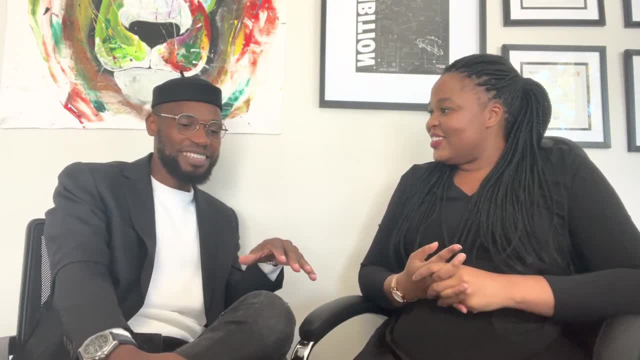 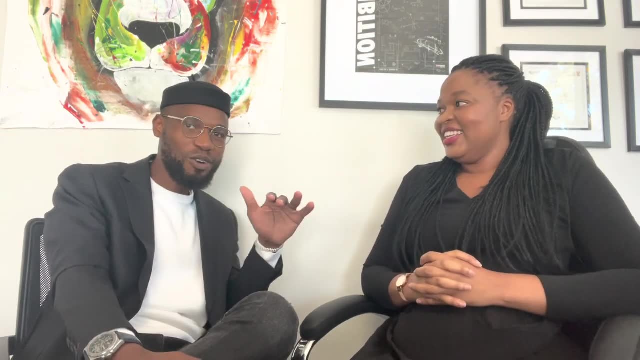 It's called Because this boy is saying things that used to make sense to me Back in the, when nobody could talk, could hear me. Jay-Z was like that's where you're wrong. I came to this game hundred grand strong. 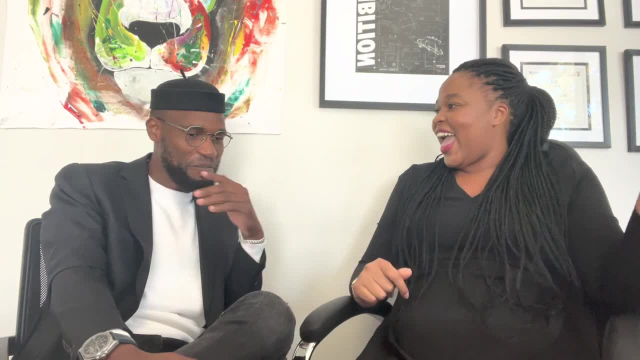 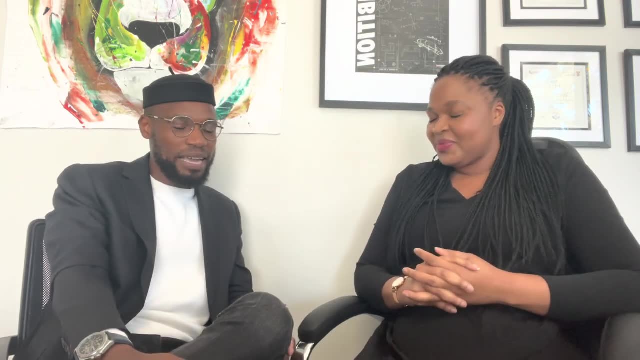 Yay, Trying to be exact from back. All right, You know what I mean. And then he was like: but one rhyme could beat that or whatever. So my definition of who I am and, as you can see, the growth is what Jay-Z speaks about. 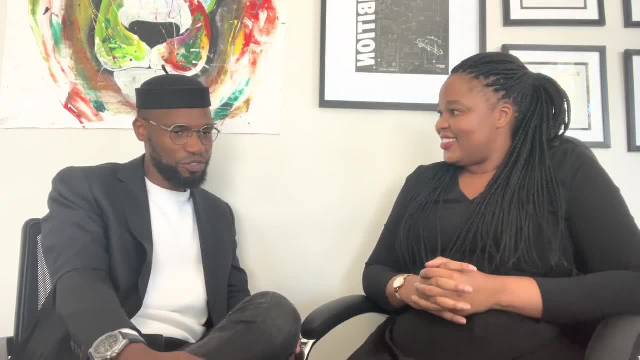 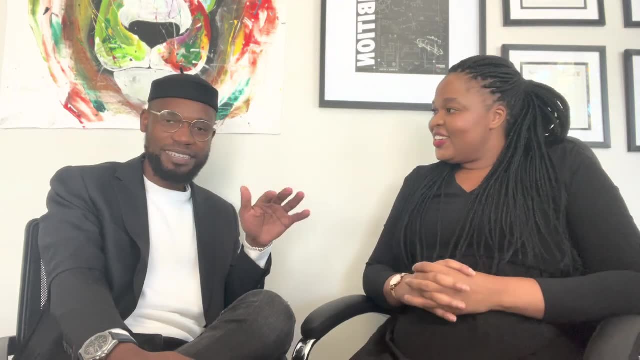 the blueprint. But how I would get him now is I would use Nasty C, this song in particular. he raps very nice, Oh okay. Yeah. they say We are keeping you in Africa. I like you girl. 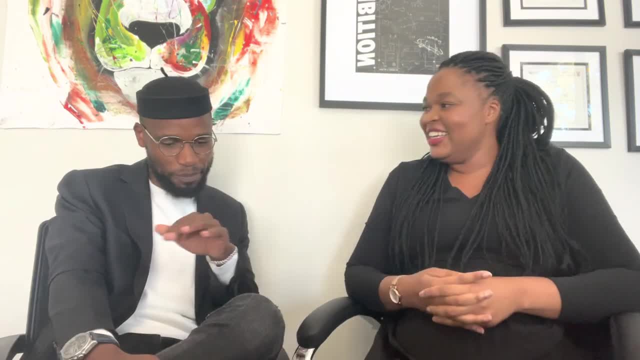 Yes, yes, But I would keep it on: Nasty C's best, Nasty C's best. Why do you like that verse? What's that line that kicks you? I think his flow is good. It's not like I'm buying into the message on it. 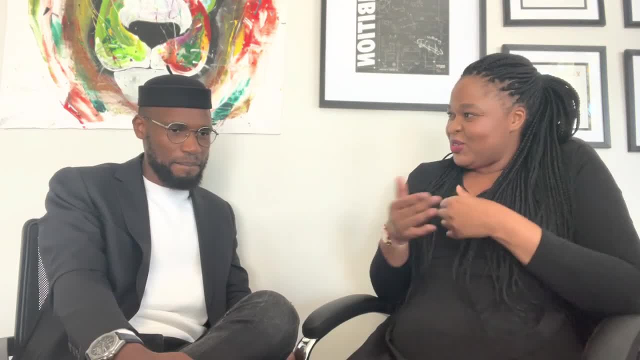 I'm just liking his freestyles and he's also from local. Otherwise, I'm selecting the better one. I'm going with better boy. We're going to bank on it. Oh, banking on it, Mr Banks. Yes, 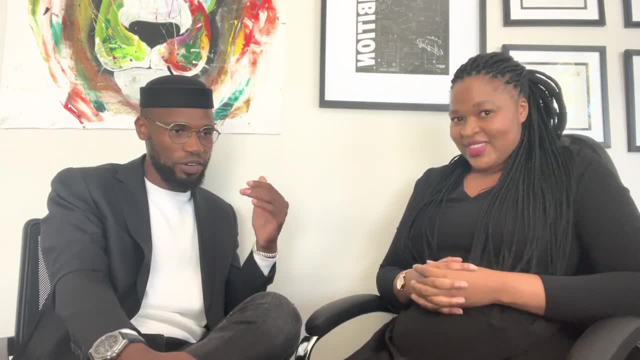 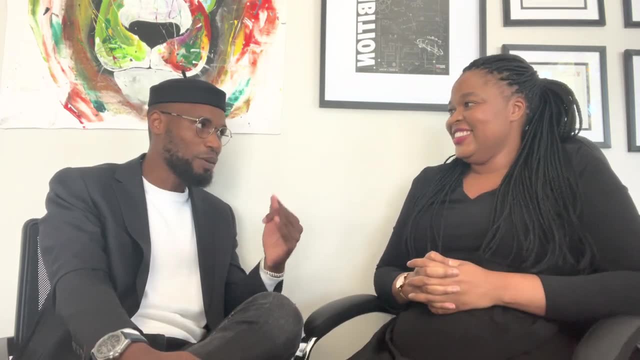 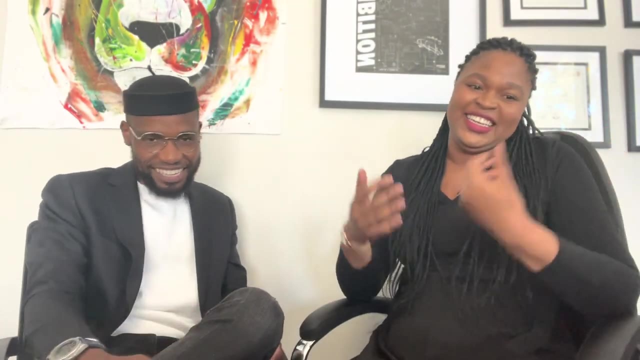 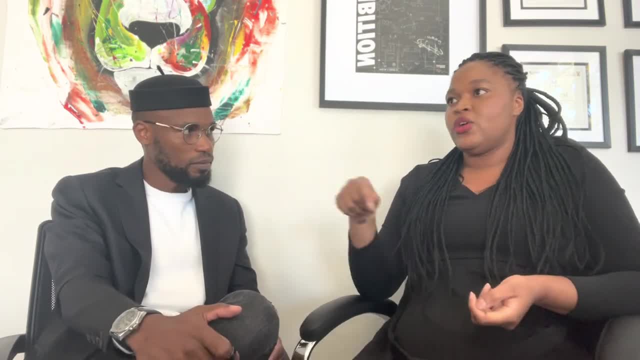 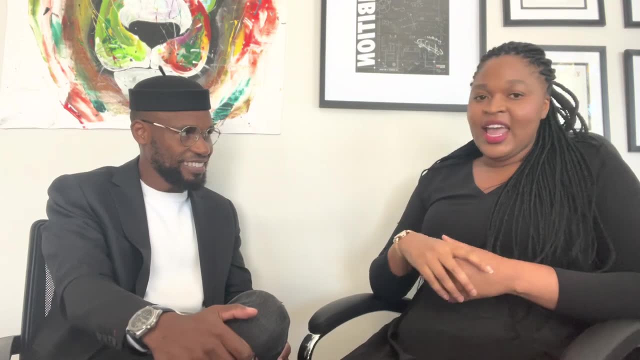 Yes, okay, you know what? what you just touched on, i really like it because i don't know, i have a problem with motivation. like motivational speakers, you should do this. you know, like i have a problem with that because i'm like sometimes you are going through the most and then you're listening to a 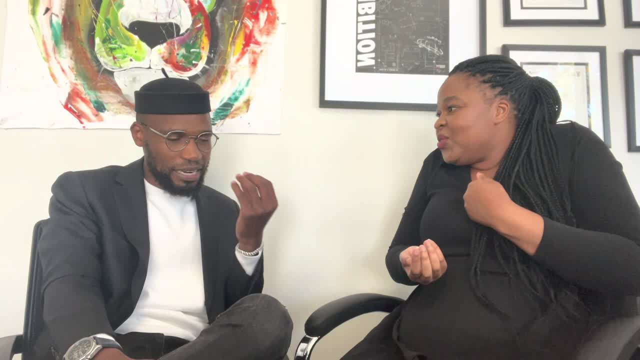 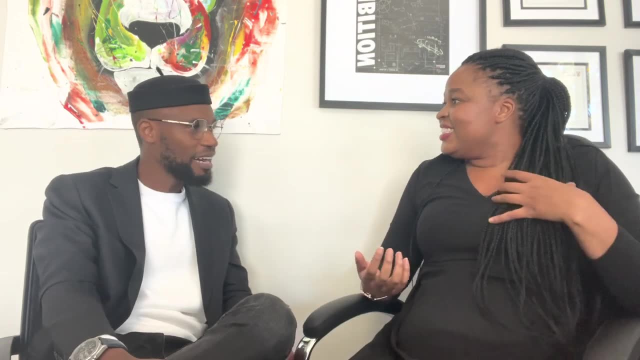 motivational. there's no substance, there's nothing, it's not touching you. tell me what to do. yeah, hey, you're gonna make it exactly. yeah, i know it's good, but it's not enough. yes, and if and when you are going through the most, at that time and someone tells you that you're gonna make it and 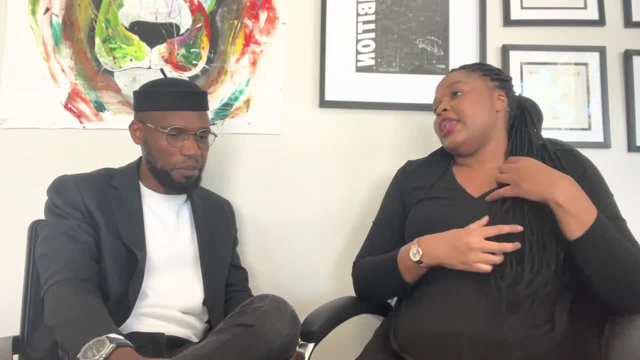 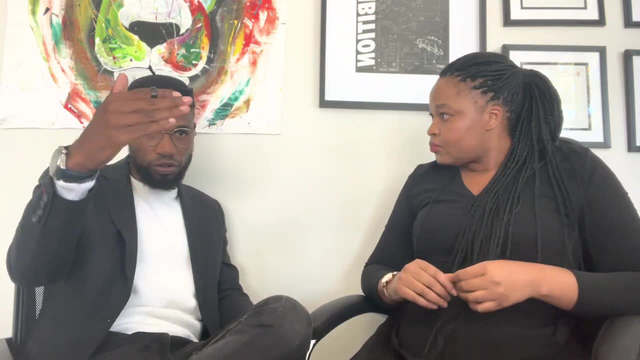 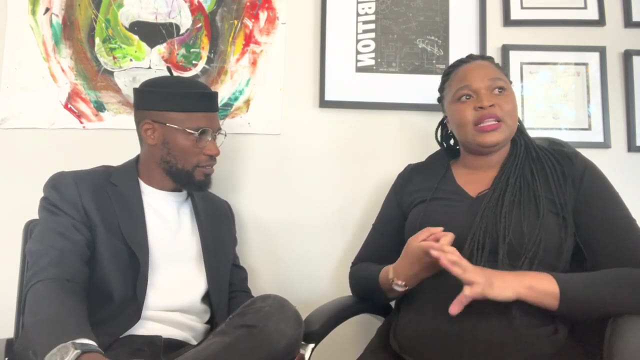 you are looking at yourself and you're just like you know, yeah, i, i think my life now is becoming that in the continent. would you agree that? pepper still looks at me and like, if you can do it, i can. i can also do it. and considering where you come from, considering the things, because in the math, 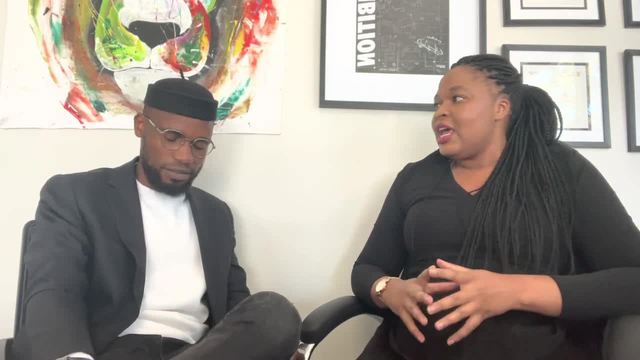 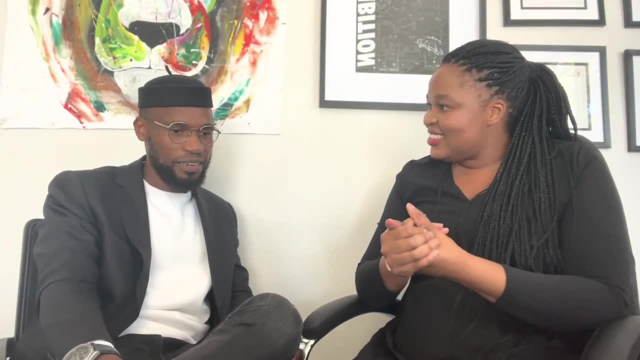 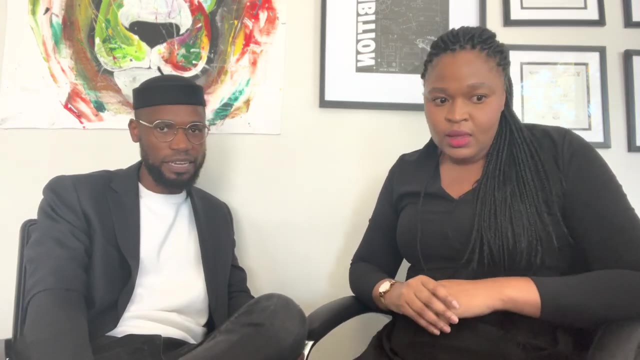 stats industry, like people go for data analytics, and this one is more basically on tech. it's tech, it's only software. so data engineering, data science, all guys are full stack. if you can get a chance to meet the full stack guys and the software engineers, you see it's proper tech. oh, okay, okay, um, what what? 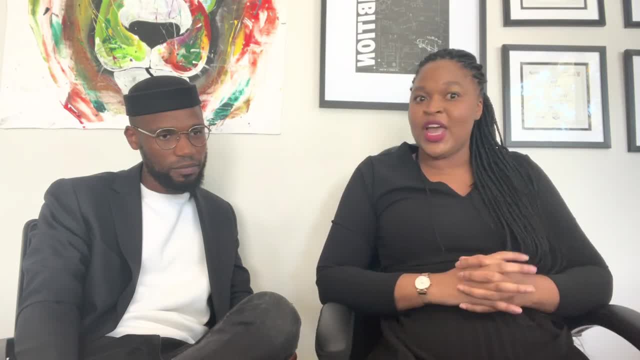 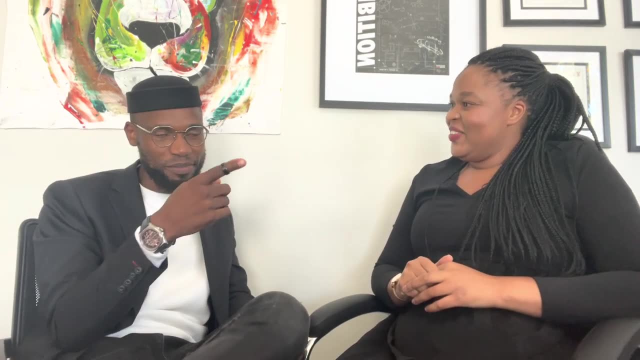 what's the last thing that you googled? if you had to check, like something, what's the last thing that you googled? i, i, this boy was here, this boy from ui. he made me google something. now i was googling a consulting company here in south africa and i wanted to see how far they are. i realized 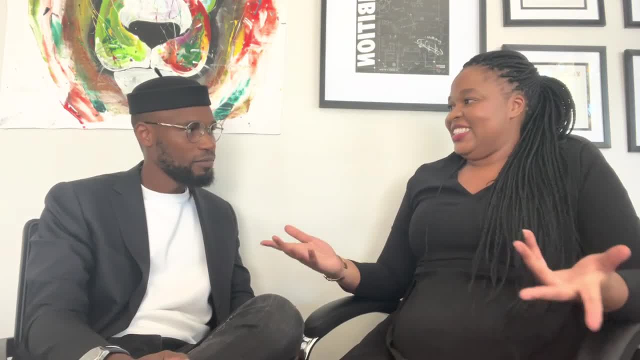 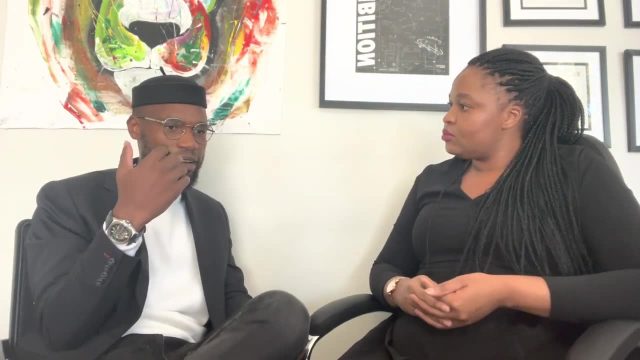 they are not far. oh okay, so you are still killing it. so you are. just. they're actually doing some things. but we in data science, many companies can say we do this and we are better than them, but they don't have a voice. that's us. they're not penetrating large corporations. it's us. i can name. 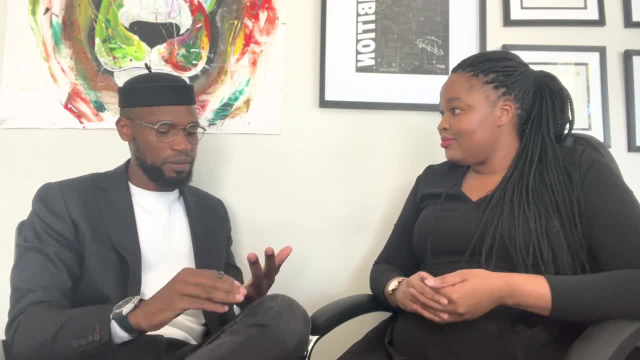 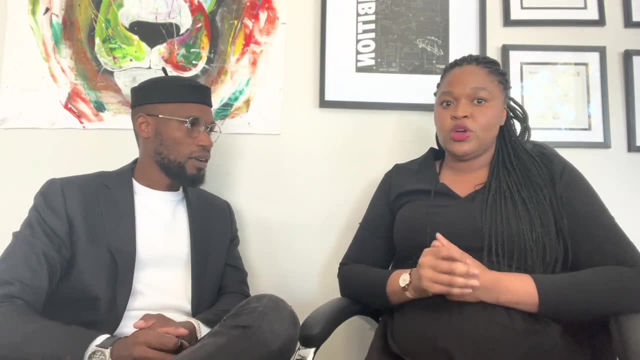 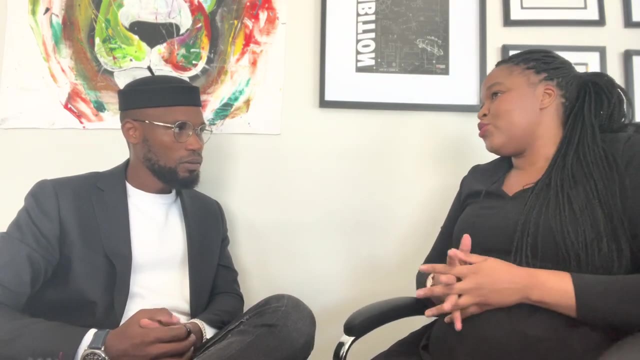 some of the corporations we're working with: dbsa, ppc, saint gobain. now we have some communication yo and mtn. to be honest, like i also, like i'm, i'm into shares and everything mtn is actually doing so, like they always do so. so the fact that you are also part of the telecommunication, yes, because 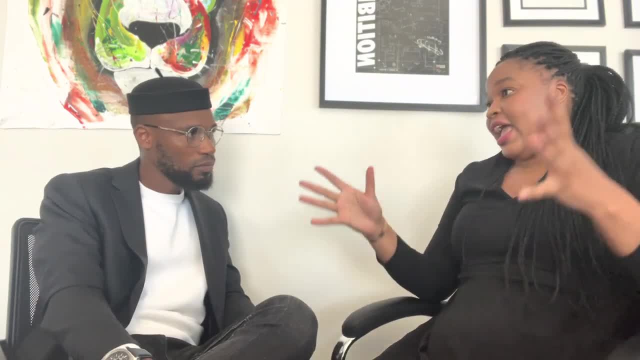 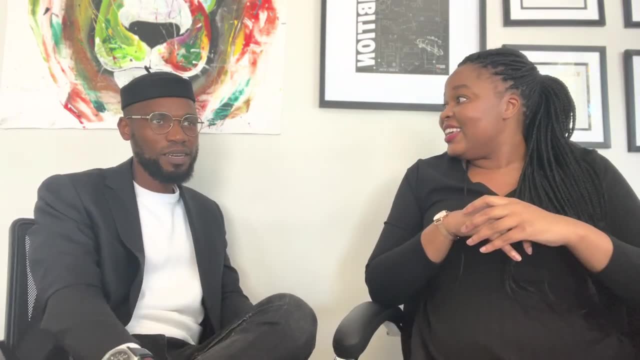 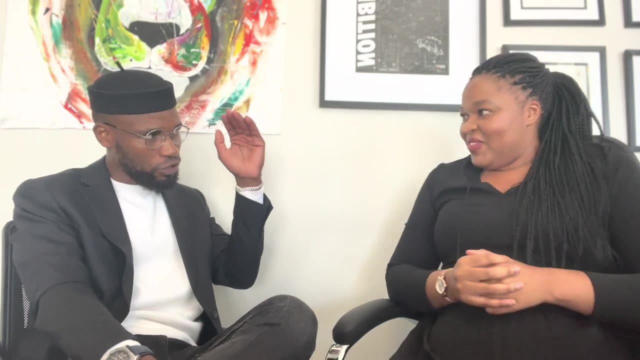 also um the telecommunication in essay and tech that are mostly the the most biggest tech companies in in essay. oh, they've got a comment: yes, they are the ones that are not. you know so the fact that you are, yeah, yeah, top level, top level service, not, not, not just not that it's top level, whatever. 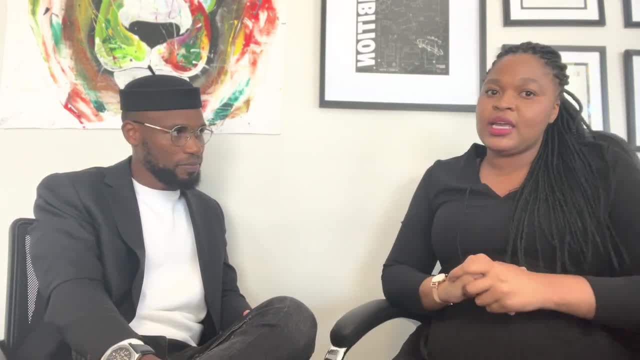 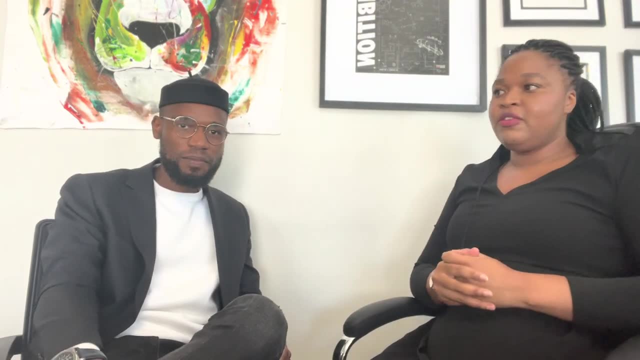 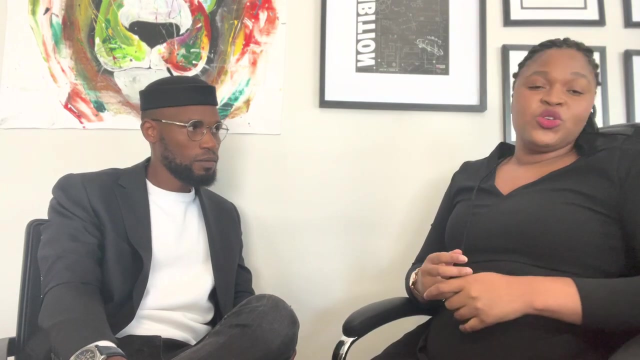 they're doing in top level. wow, i'm so inspired. guys, um, this is like i don't want it to be a longest video, yeah- but also i'm so inspired that, even from a bsc mathematical, um statistics- you can literally go and you don't. you can go and start your own thing. you can make sense. you can make sense out of everything you. 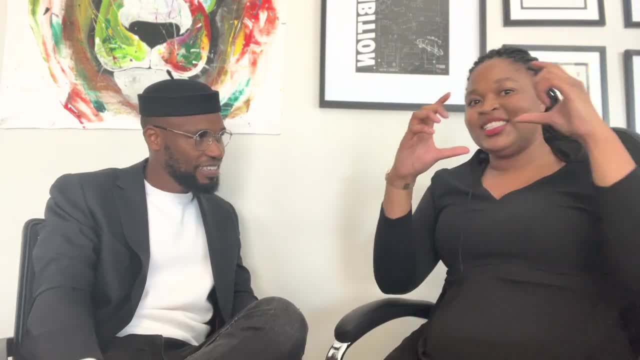 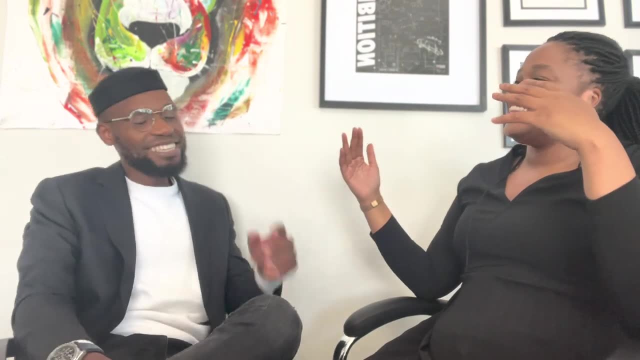 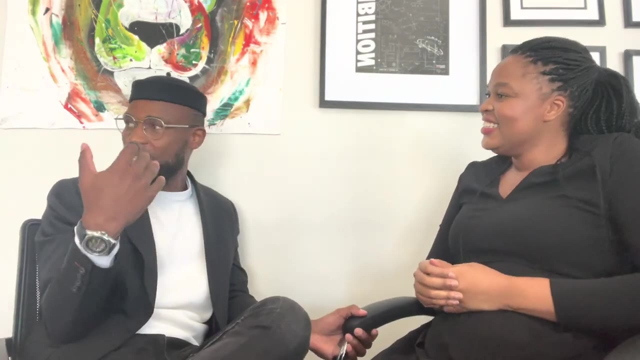 know, and you know what i also like. i'll also insert this on this. i liked that mathematical thing when you get inside, i just knew that people like you will hear me. you know the language exactly. i constantly say this because the people think mistake us for advertising. i'm like 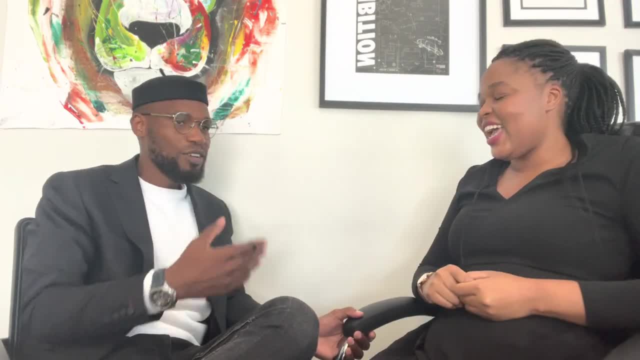 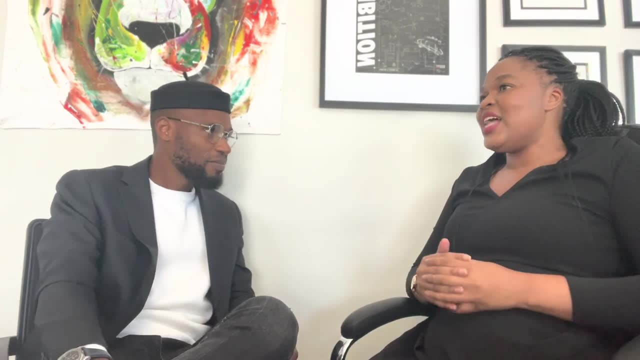 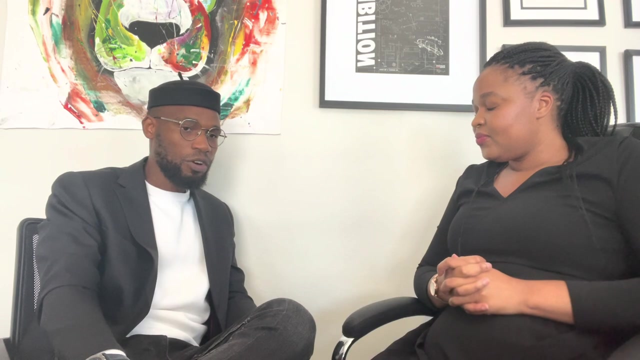 we are mad people. yeah, we speak in numbers. yeah, so there's no other language we understand except those four minutes. yes, that's beautiful, yeah, so what's what's the theory behind it? well, the theory behind it is: um, i think there's a lot of um. god has created so many things that 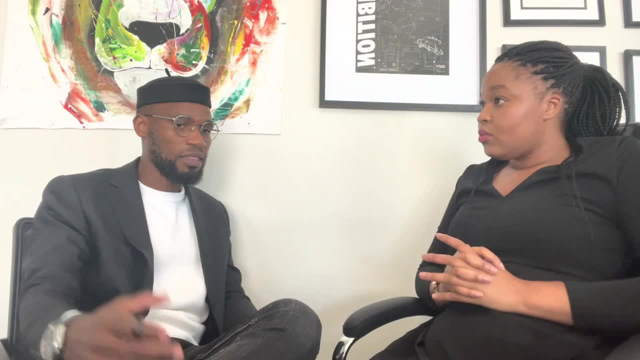 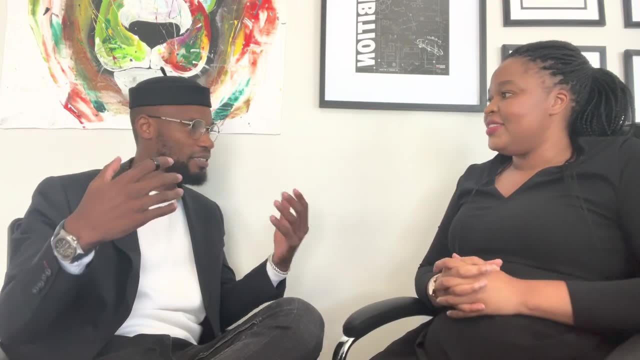 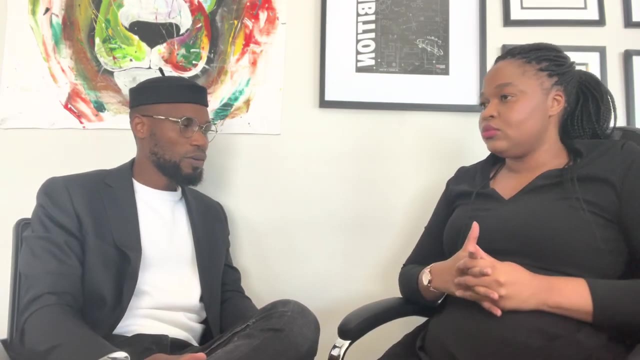 still can't explain. they are beyond understanding even the pyramids in egypt. they're beyond understanding. what we should be creating should be beyond, beyond understanding, and that requires deep learning of mathematics or deep learning of science, you know. that's why what we are building here, these are we are working with global billions and corporations. how is it? 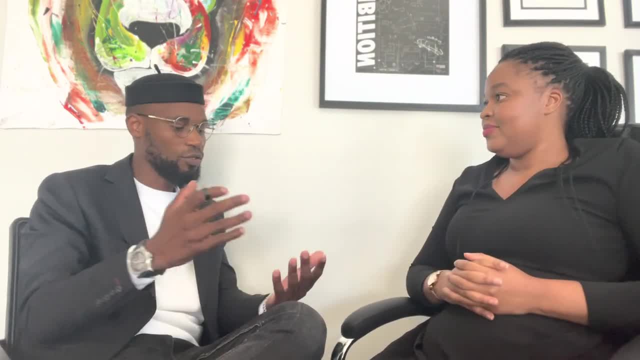 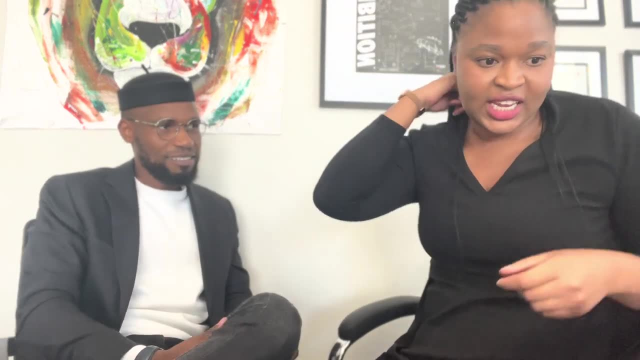 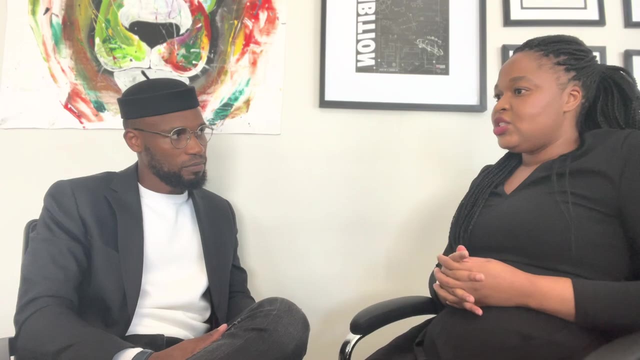 that we can multiply them because we have got company in the us and company in the uae. oh, wow, wow, this is. this is actually great. um, so were you actually doing well in the corporate industry? um, in a sense of where you were working before, where you like, maybe managers or, or you. 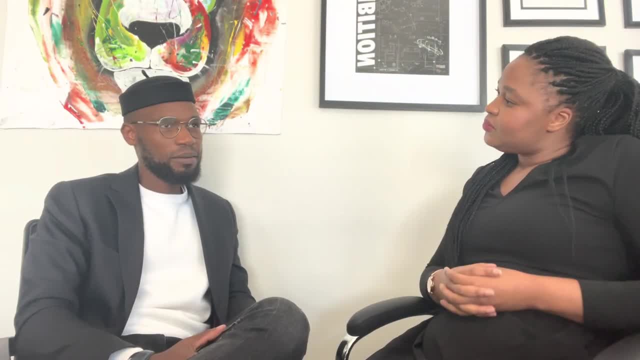 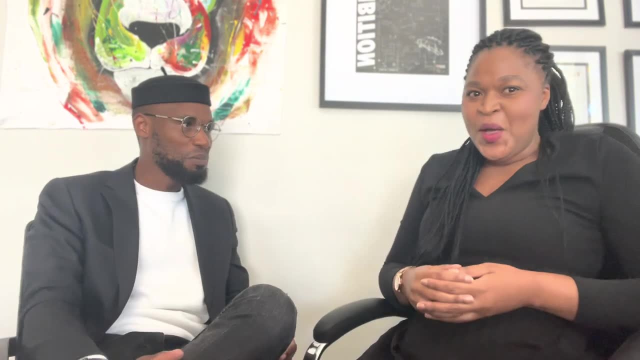 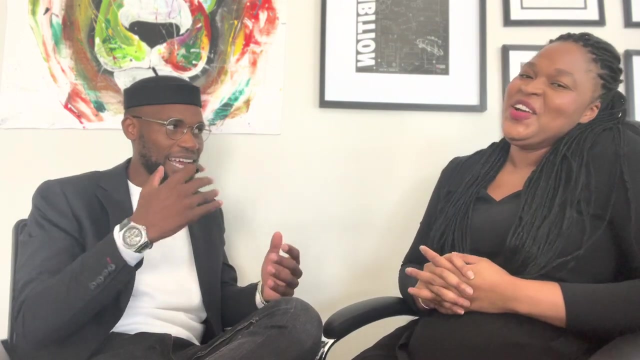 were just doing. i was just a nobody. they didn't understand me, but i was obviously. you can hear my voice, i'm. i was rumbling, but i remember i used to argue with buyers. i have you with the enemies, i, i was the person who hold the show. nobody can already show like i. like i can argue because i. 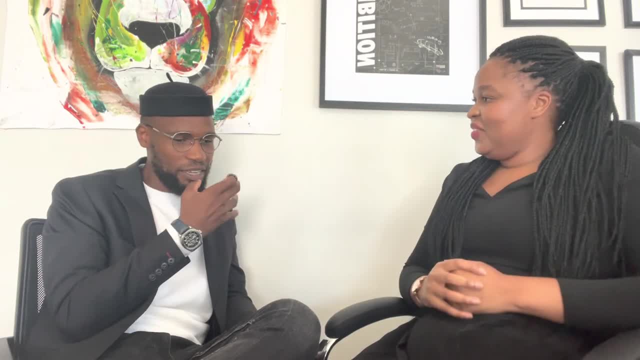 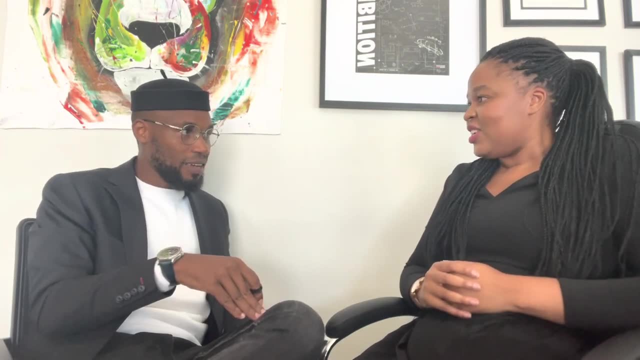 don't mind my stuff, but i'm arguing in the wrong. it's like i'm an eagle amongst chickens and i'm talking about flying. i'm not saying it in a bad way. i mean no, no, you should say it with the chest talking about how possible it is to fly. i've tried it. i've seen myself jumping more than what you guys. 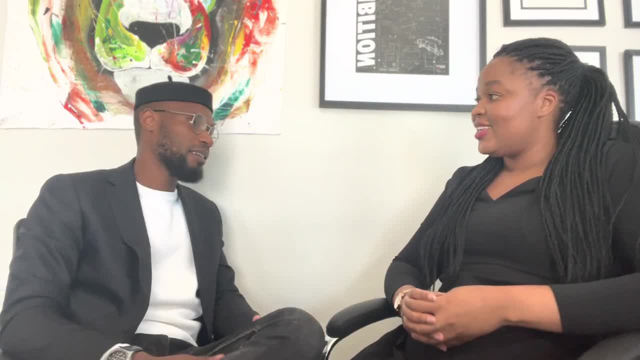 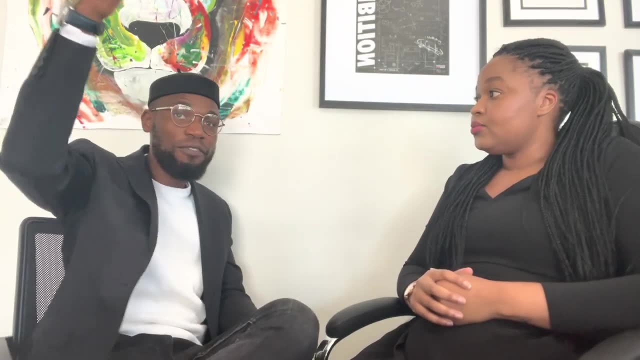 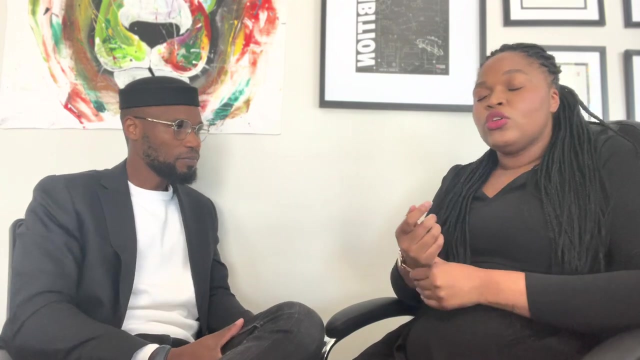 do and it's possible to fly, and everyone in there is like: man, please stop playing, man, nobody can fly here. if you fly, you reach here, and i'm saying you can fly higher. and they didn't believe, so i had to leave and now we're flying. i can right now i can work with all of them. yo, that's powerful because 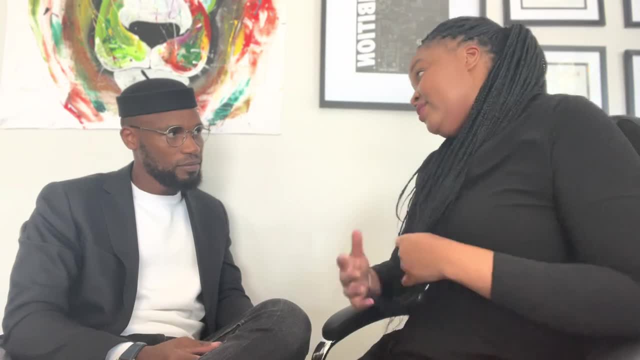 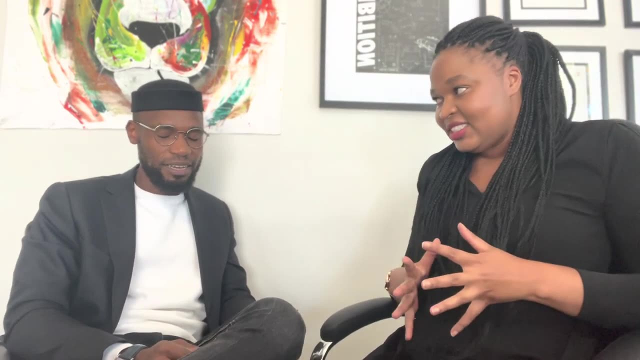 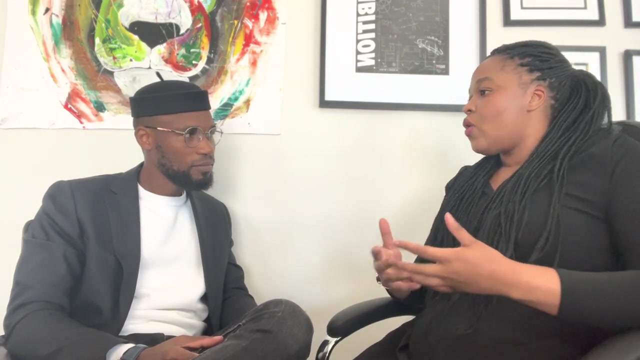 that's the thing about the vision that i i believe in god. okay, oh okay, oh okay. yeah, i believe in god because you know sometimes it's so hard, yeah, you know. but uh, god gives us the visions and normally when you have a vision, it's so hard for you to. 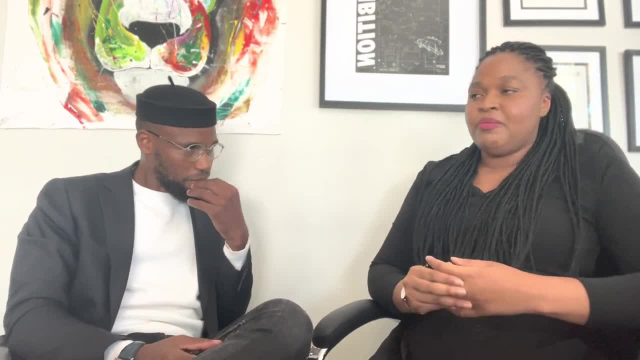 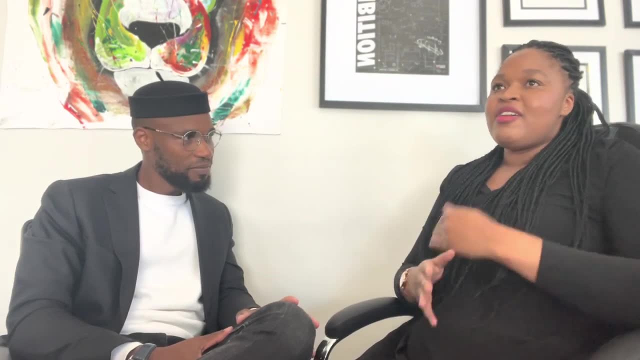 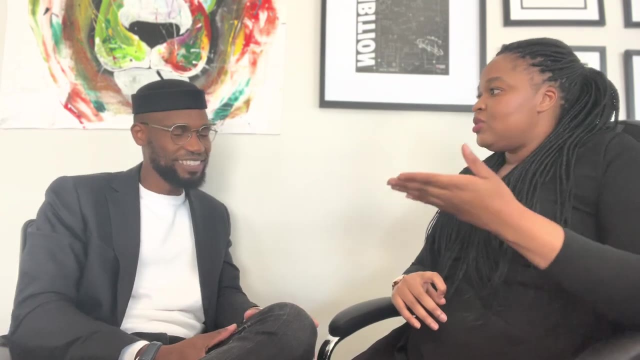 interpret it to other people and tell people and be like i see myself doing this, you know, and having to explain to your. that's why i never question people's questions, because now you understand that there's a vision that you have, but now when you try to explain it, no one doesn't. 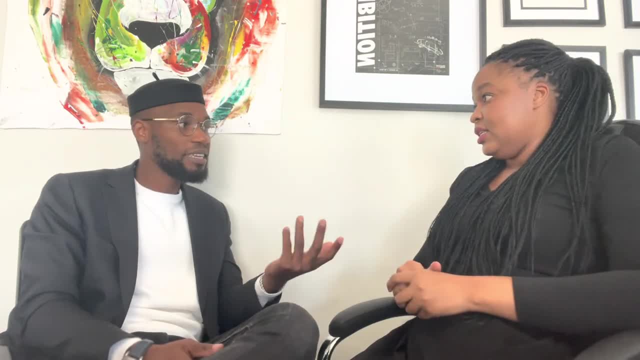 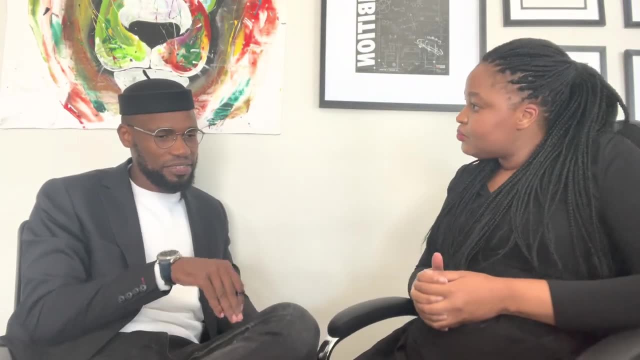 make sense. it doesn't make sense to yourself, yeah, because you're not living in it at that time, at that time, and you're just trying to work to connect. it's blurry, but i can say that that's what it's like in my life. so i've been there for someone else that i've never seen. 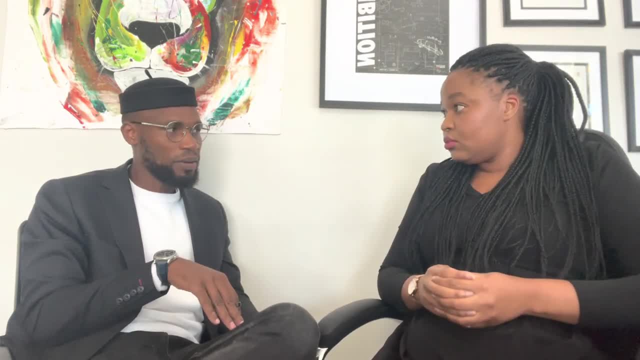 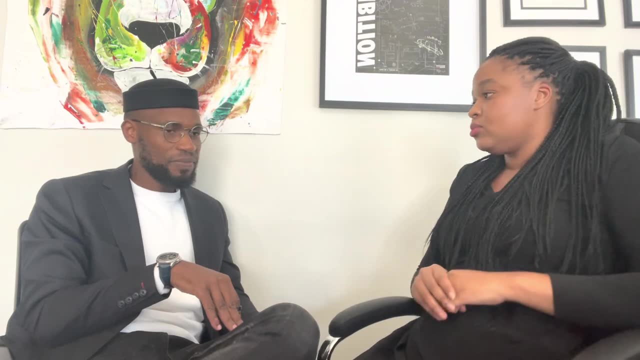 before. and it's the same thing with the things that happened in my life, because every time that i've taken any kind of step, i've never thought i'm gonna take that step, because of the fact that something happened the moment that i took that step. everything that i've said in those rooms 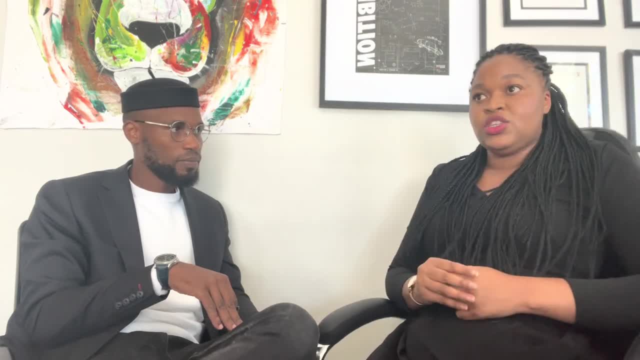 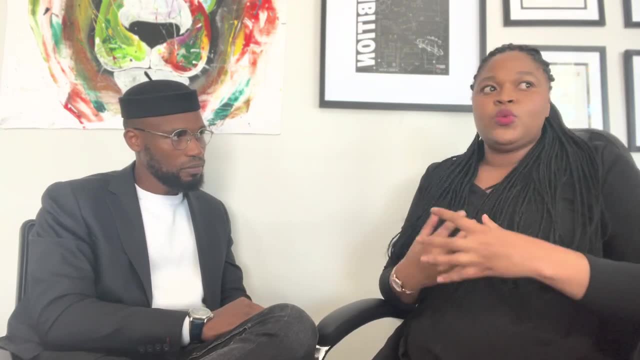 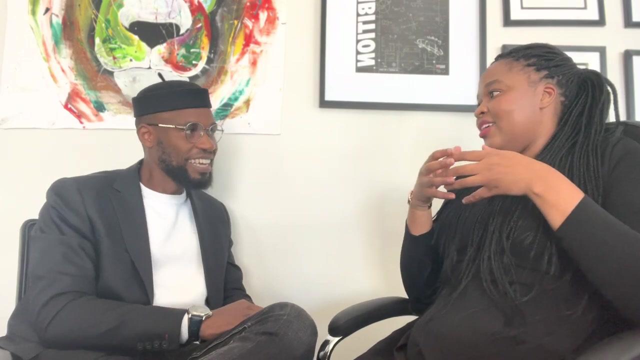 everything happened, even 10 times, 100 times, because nobody thought i would make it this far. and now i work with some of the largest, largest corporations. enough to just go out there with the vision that you have. you have to start somewhere, you have to do this the right way and it's good, and you learn there, you learn there and you and. 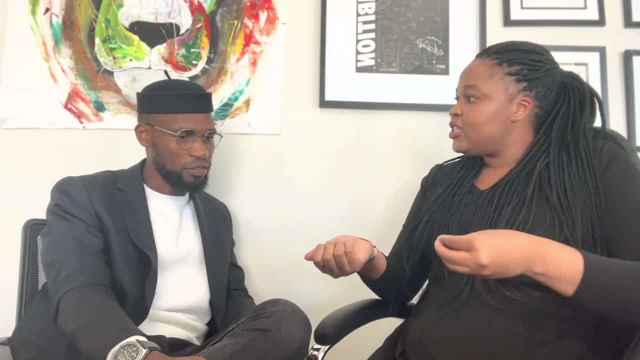 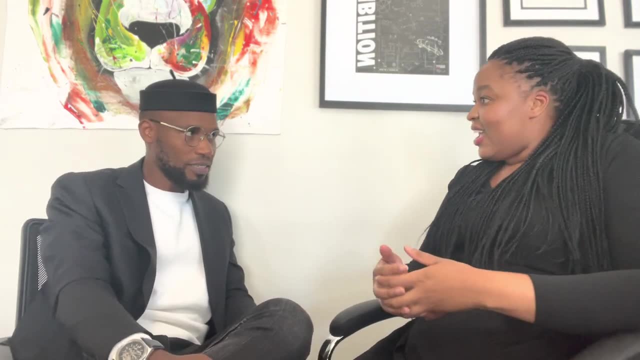 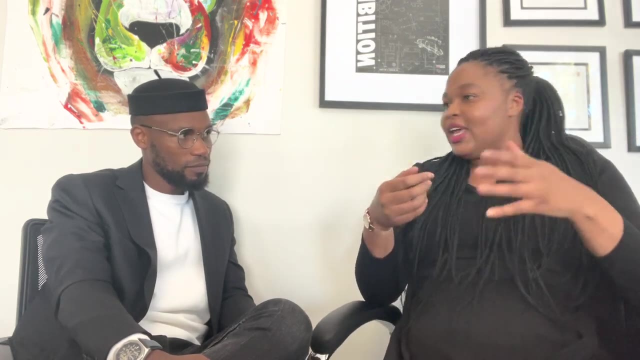 i like the fact that you are also appreciative of the fact that when you were there, you could see that, okay, this is this. you wouldn't figure it out outside, outside. you need to be in there so that you get to see that it's easier for you to see actions and like having to research it for. 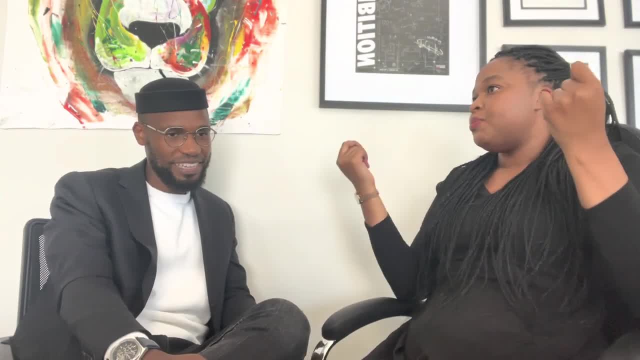 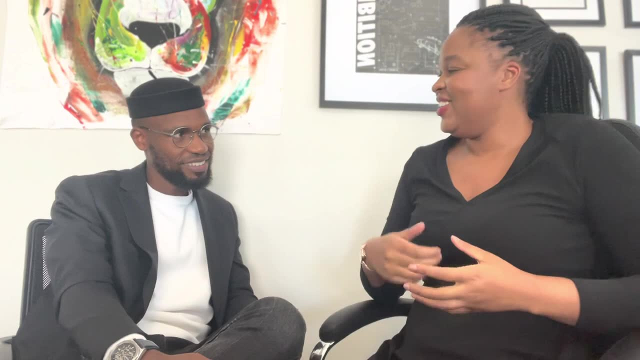 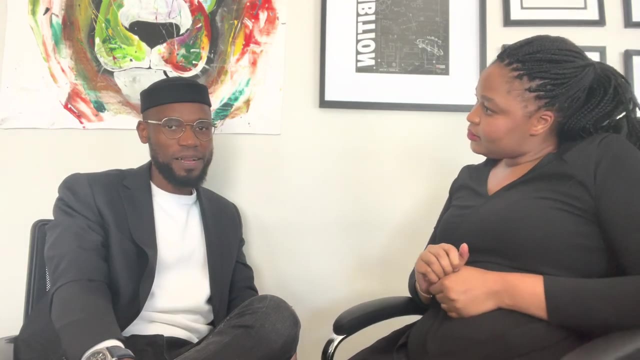 yourself, and that's one of the things that i think i'm like that's powerful. you know, that's really powerful. um, um, so, how long? how long? how long? okay, thank you. how long did you build your company? five years to be a multi-million- uh, multi-million company, four times award-winning in technology. 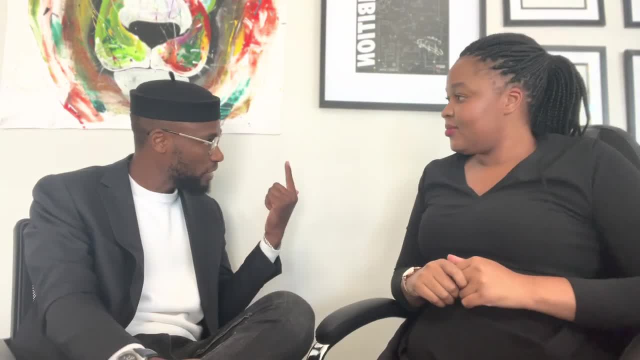 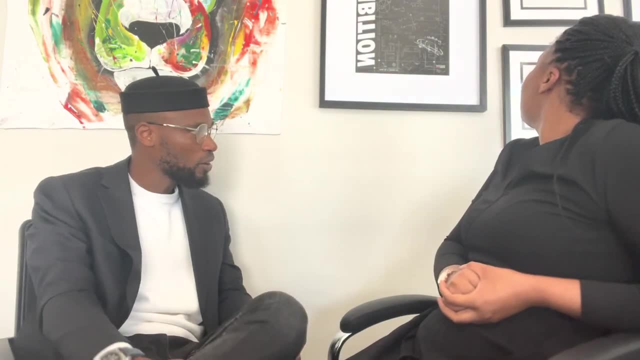 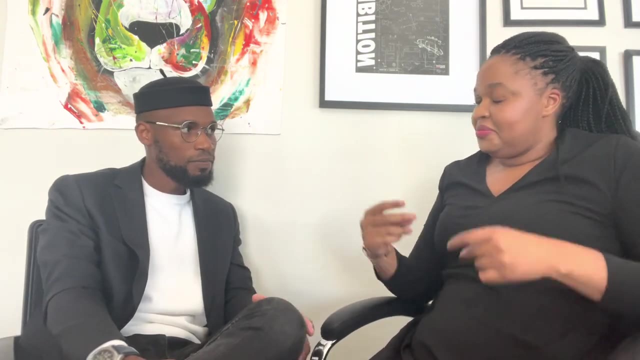 in innovation, okay, and um, in department of science and innovation, ministers award for overall excellence and, uh, we've got a different style of management, so but, uh, we want also management of people. now in may, we are in the category of africa tech awards and top 10 already in that. 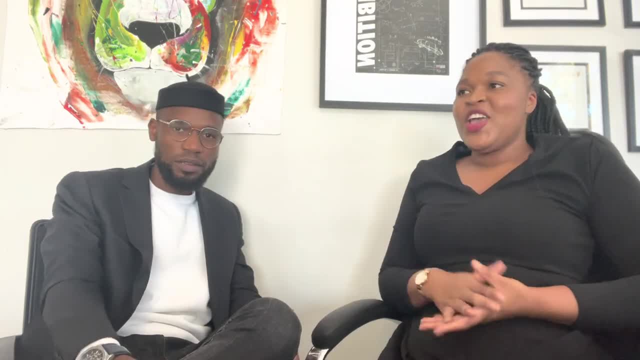 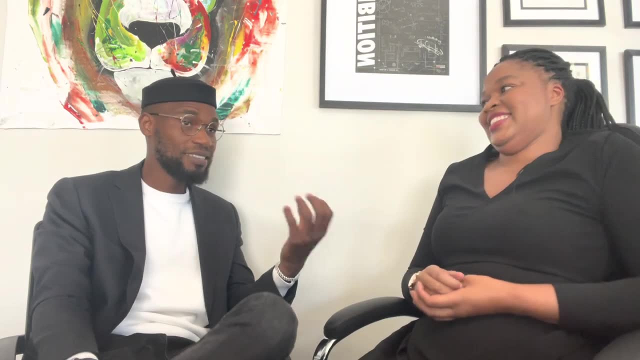 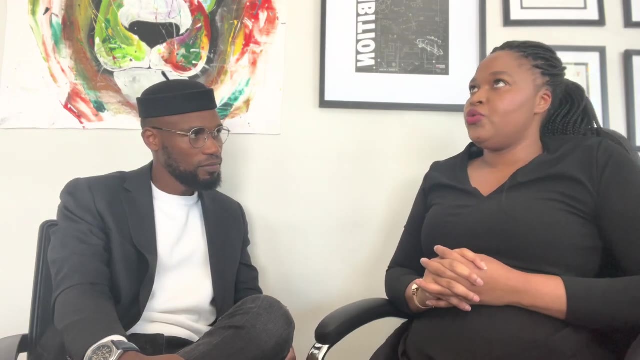 so i'm hoping you heard it yourself, guys. you really had it, for how do you, how do you get to a level where we were talking this with people and they couldn't hear it? yeah, and now they just see it to witness, wow, wow, that's one of the so, um, obviously, uh, you had to go through. 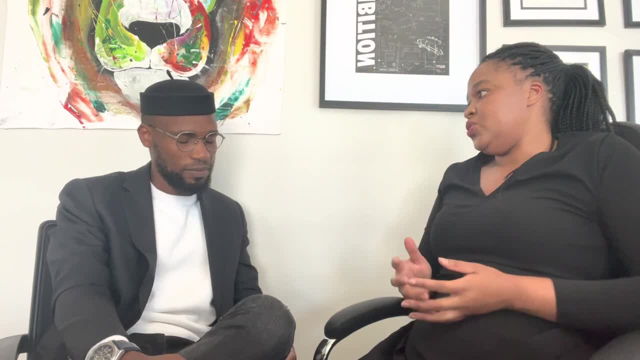 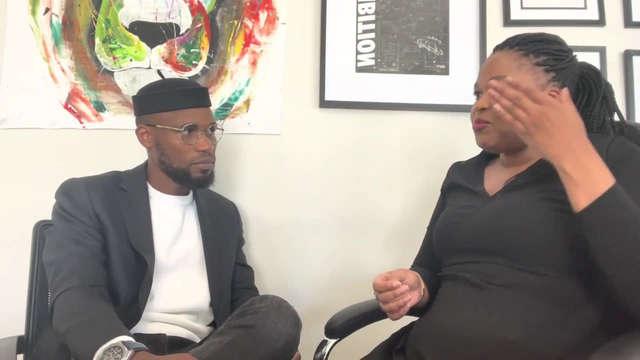 like: obviously, when you were building this, no one understood you. you know everyone. everyone was just like: okay, and you have this thing in your head and it's there every time when you wake up. it's there, it's haunting you. it's like: yay, it's with you, i'm here, you know, um, did you leave uh? 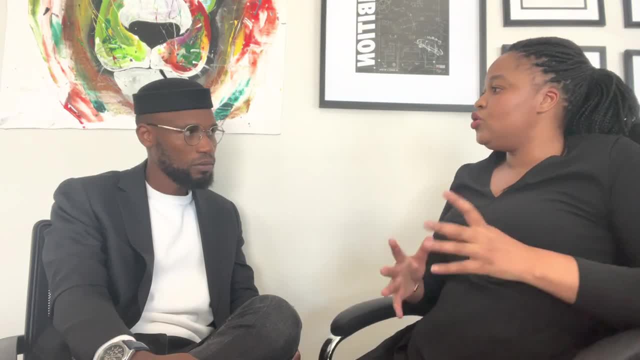 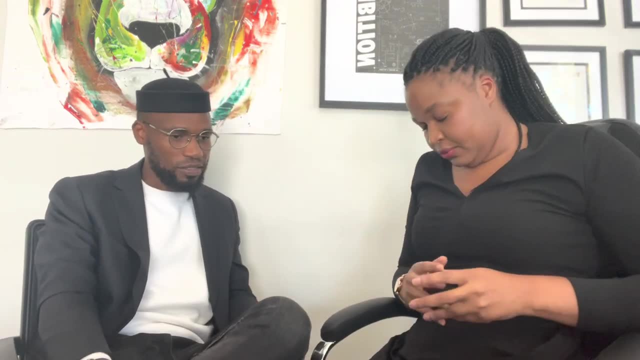 corporate completely, or you just felt like you know what, let me do this on the side and you're, you know um, i'm from, i learned from stats and we learned some. we did some econometrics and they say: you always say don't put all eggs in one basket. but i've tried to not put all the eggs in one. 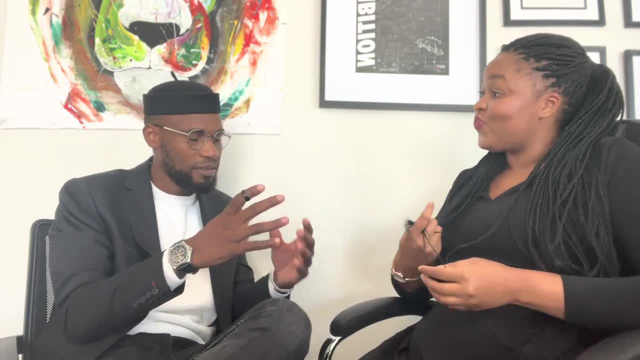 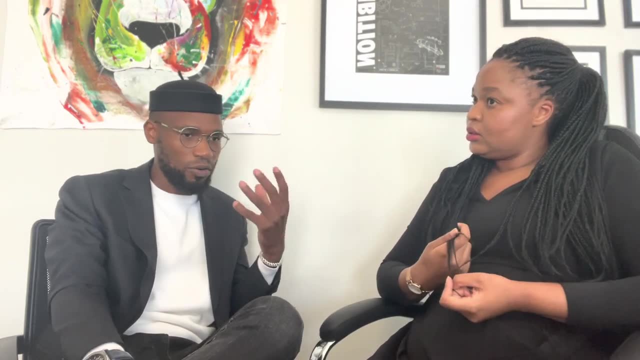 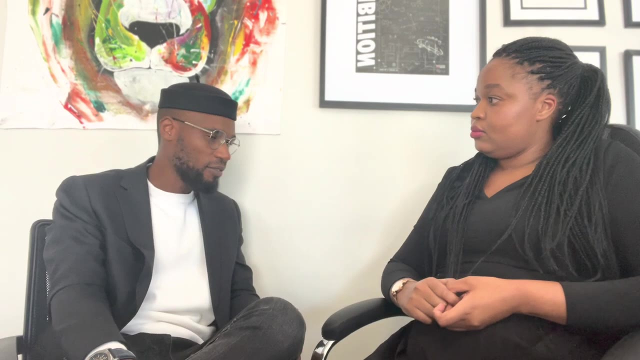 basket incorporated. it was like i'm managing nothing. i went on it 100. but the main reason why i went fully in and i never thought of corporate, i used to get calls. network finance guys say they want to what position? i mean this agency is trying to bring me back. i never, never. 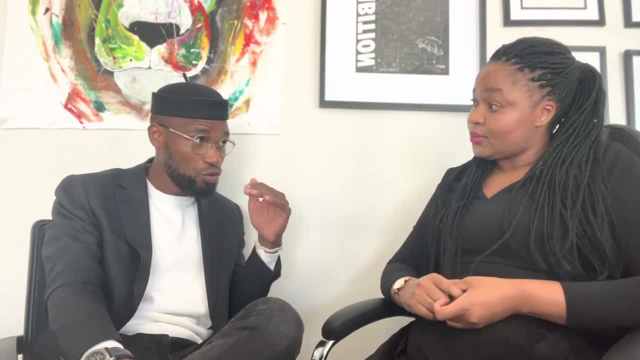 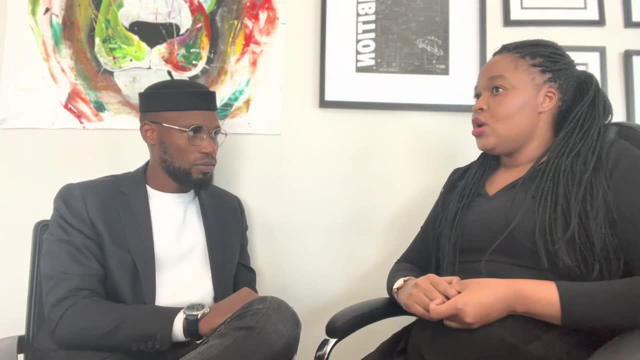 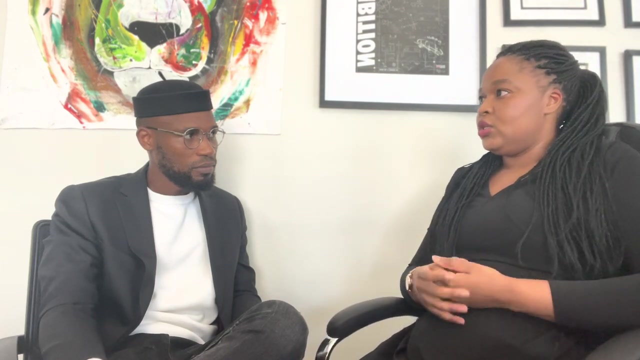 blinked to go back, even when i was going so hard. i went through so many painful things, but i trust, i believed in me. i know what i can do, so obviously at that time there's someone who's watching who wants to do this: start their own thing. 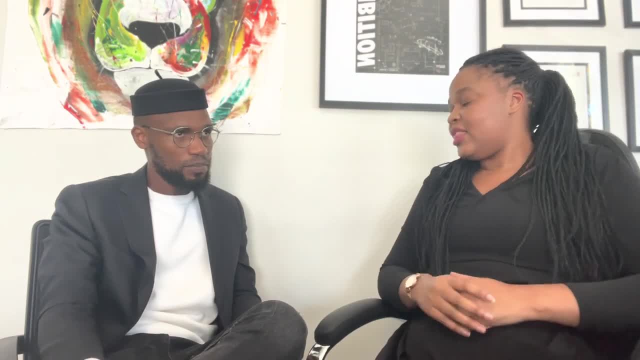 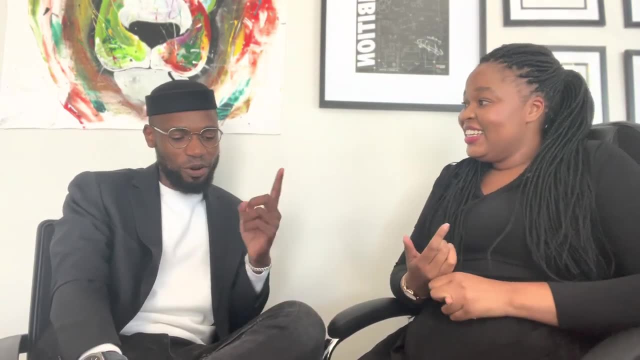 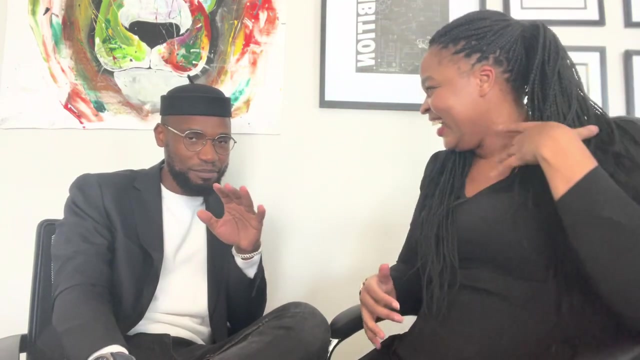 but maybe the finances are not allowing, because at that time you need to eat. but let's be practical, let's be practical. we live in this way. okay, one thing i did right: i was already married to party, so party was ending your food. the bridge was not empty, guys, so i was struggling mentally and solving the problem, but not food. 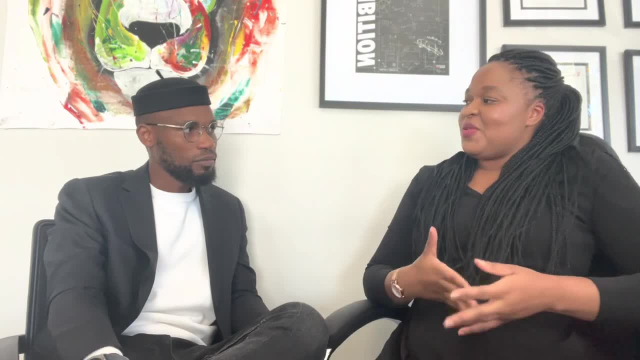 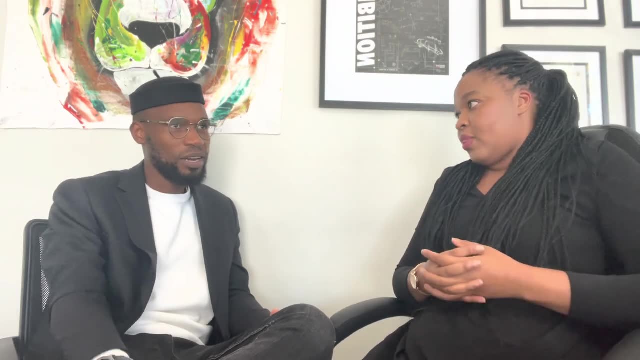 not food. okay, so your, your best financial thing was your. like, you had someone who was there for my head. if there's food, you know, you can wake up and move again. only thing, that's the only thing i needed- petrol i was. you know, i was finishing full tank every day. i was moving around. 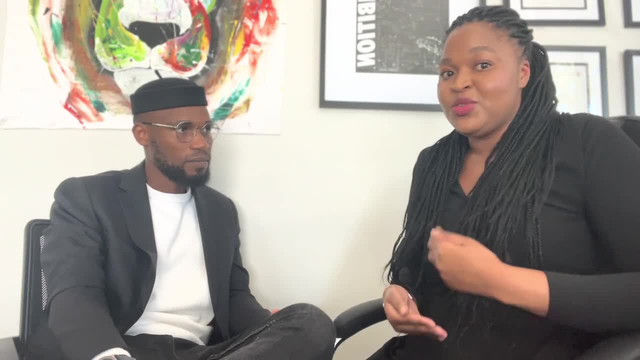 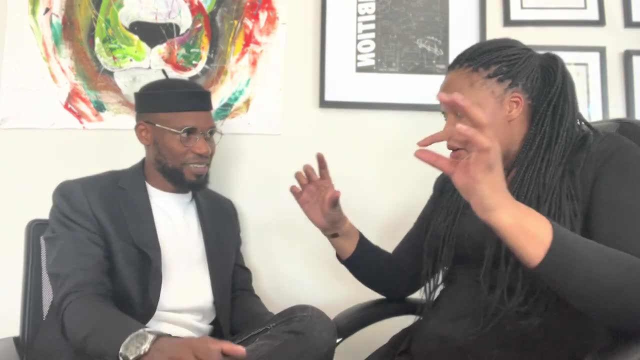 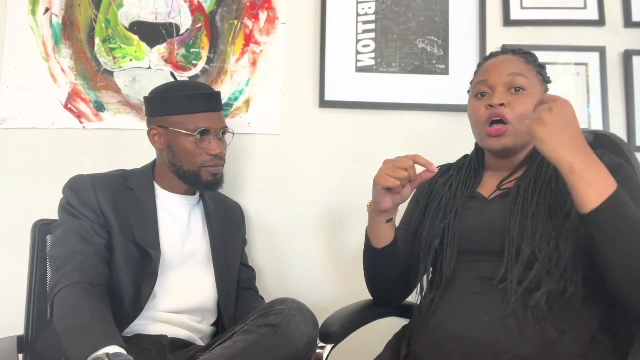 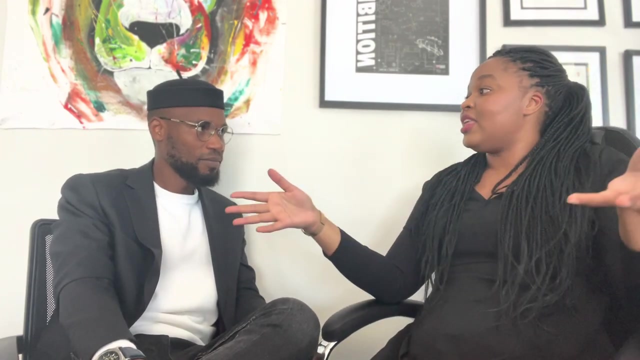 but uh, guys also just know that you have to eat, even if you leave. your color is first- and i think that's one of the things that we need to also emphasize- that solve the eating first, and then you will leave, because you can't just to, and then you are out there. 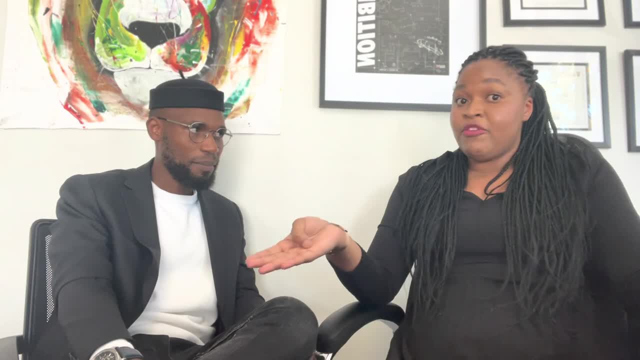 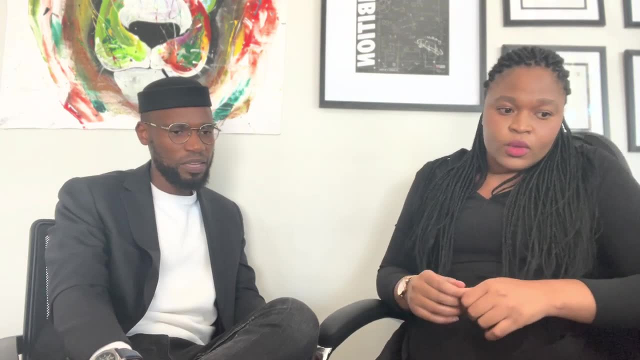 $. you don't go and you don't get out and especially if you dont have, don't come from a beg for it. wellこれは background, you don't have anyone to back you up. yeah, so the also the thing is, this is so hard that people think you are mad. you know, my, my family actually thought I was mad. I didn't have 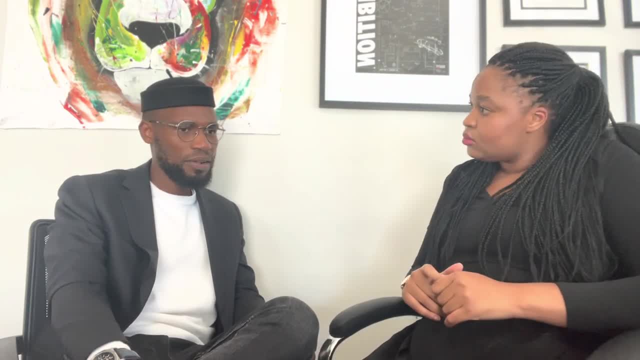 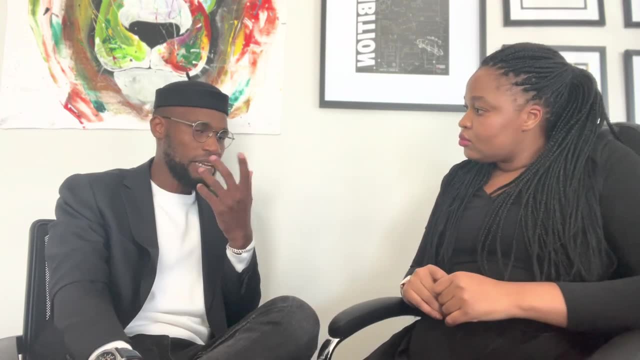 a backup from their family. they just looked at me like why is he doing this? and the only thing I needed to do was just to believe in me and I just knew that I mean I love them, but I just knew that they would believe later. now I'm proud to have put my father in one of my properties he doesn't have. 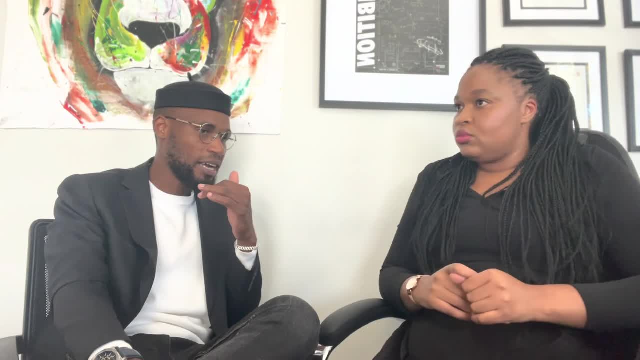 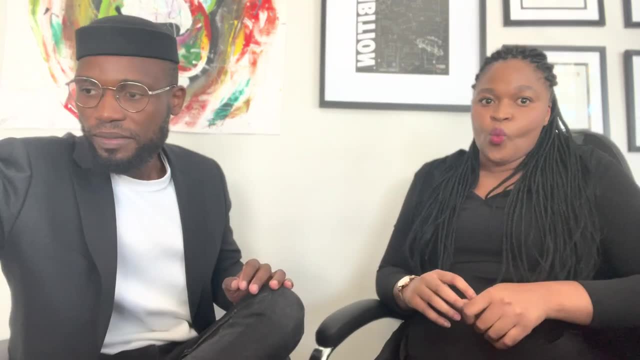 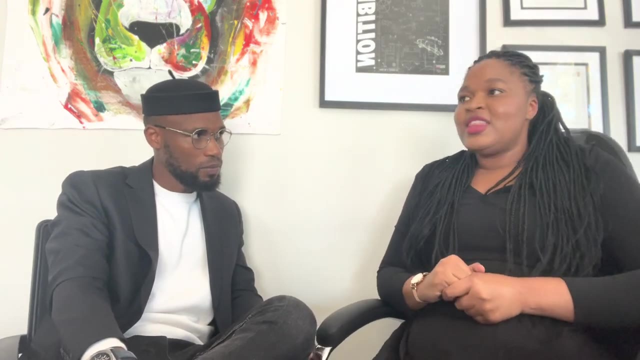 to pay nothing. everything is paid. I gave him a car. he's got his own car, but he's got a new car. he's got a nice property that a person who works in corporate- um, a person who works in corporate, yeah, and then, uh, with the networking. obviously you had to go out there because you have this. 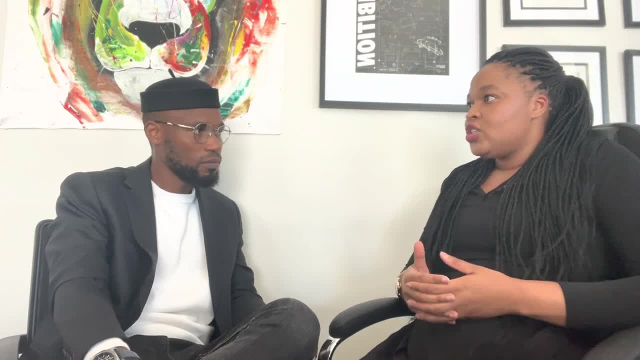 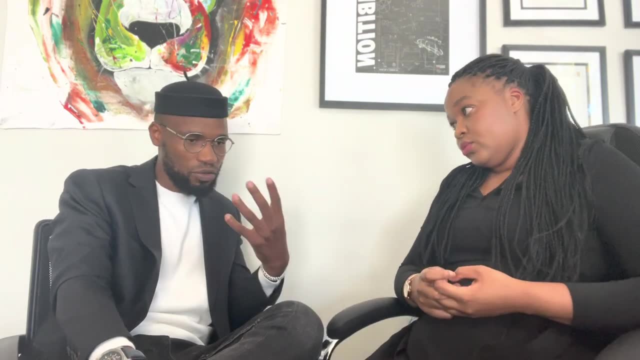 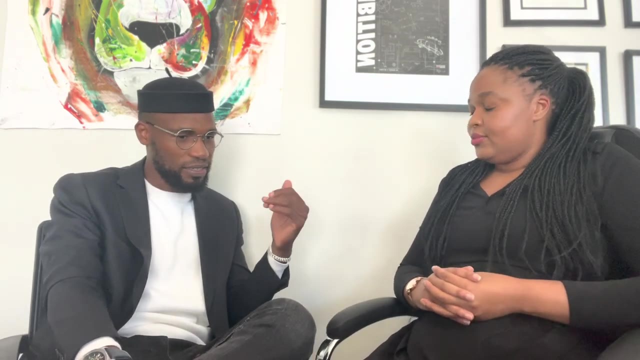 vision. you have to go to a company. you have to talk to someone, so how did you go on about it? it was there difficult data, science or whatever you're trying to use to be at the back analyzing numbers. you haven't perfected the skill of talking, so I think I struggled 2017. I don't know. I was not because 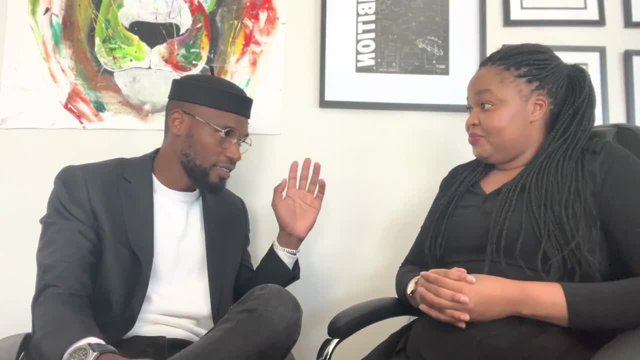 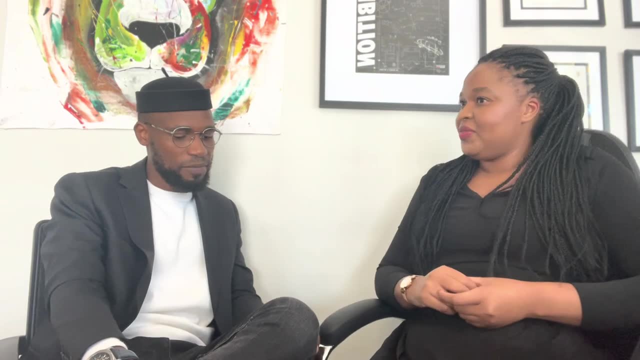 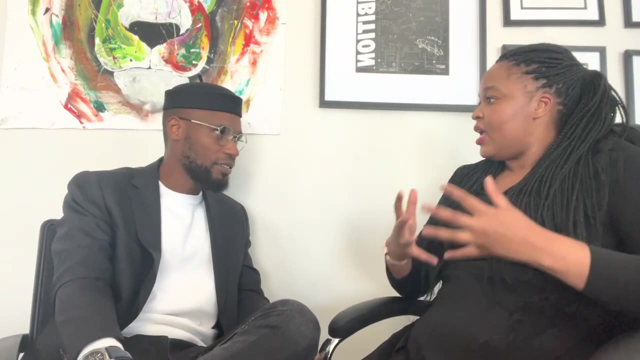 2017. I hit a deal with keyboard touch in this radio station so I was speaking well, but there was something I didn't have. like when I work in corporate and trying to get deals, it was like they reject me before I start speaking because you didn't. yeah, I understand, I didn't have it. yeah. 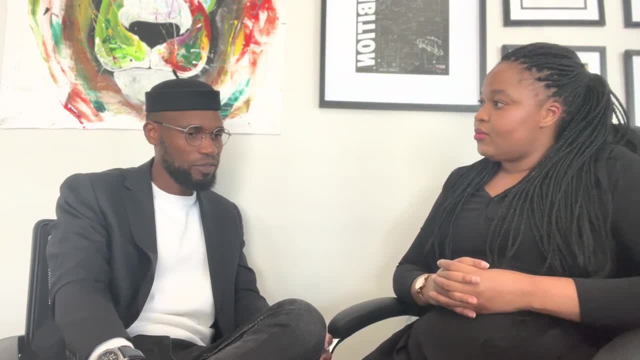 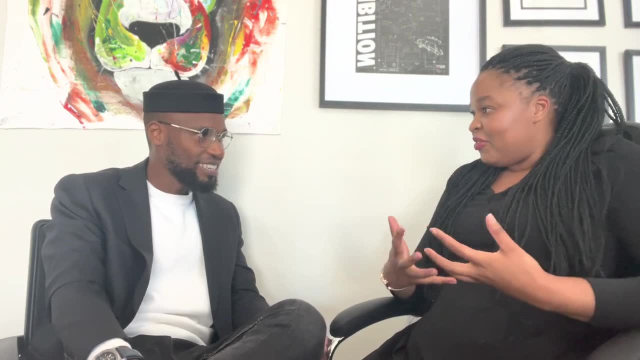 I don't know why. it's like you have to build a profile, you have to build a name, you have to be known for something didn't happen. yes, influencers would say: build a brand for your brand before. yeah, so influences that brand. but I could understand that because already I was managing in some 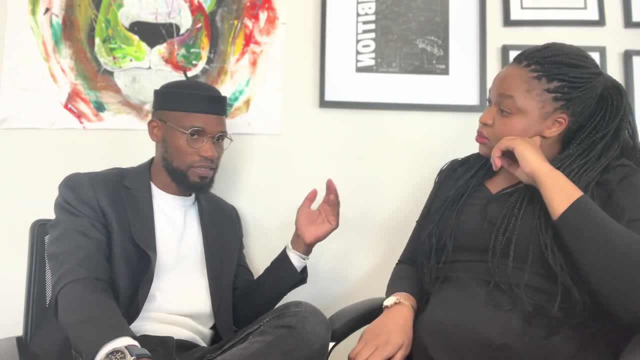 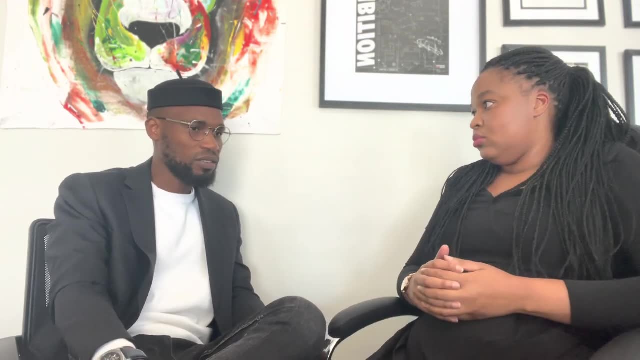 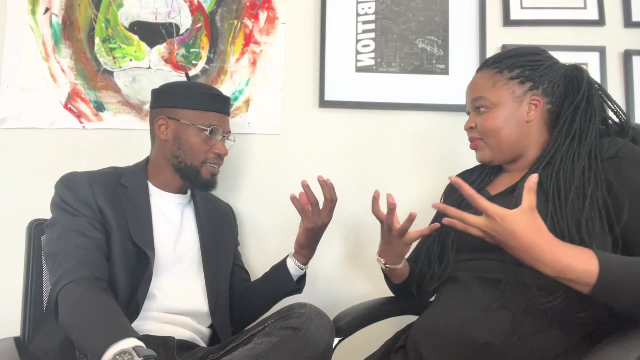 artists and Mumbai in 2016.. I was managing some top level artists, so I understood the level of positioning and brand. so by 2017, already I was. I mean, I was recognized by a lot of people. I was saying I had an interview with Thibaut Tate in 2017.. So already I was in the bracket. 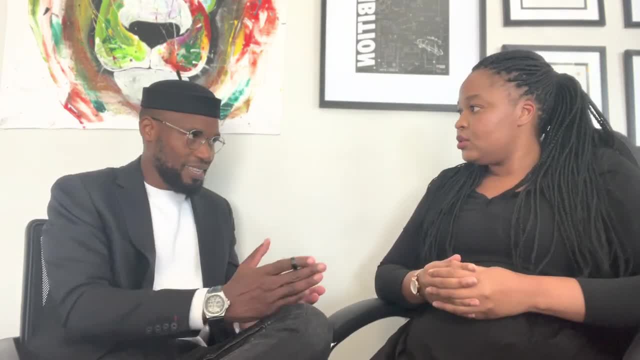 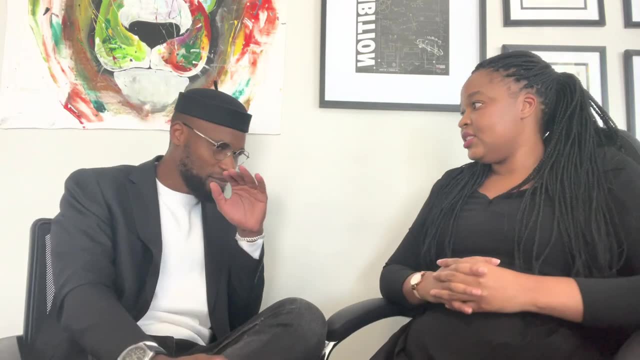 But my name was not there So I needed to build it. So, 2017-18, I'm trying to build a name. That's why you see me now on LinkedIn. I had to start now saying the Facebook, the Instagram, is not me. I had to go where me is and where I can speak. So I started building and my 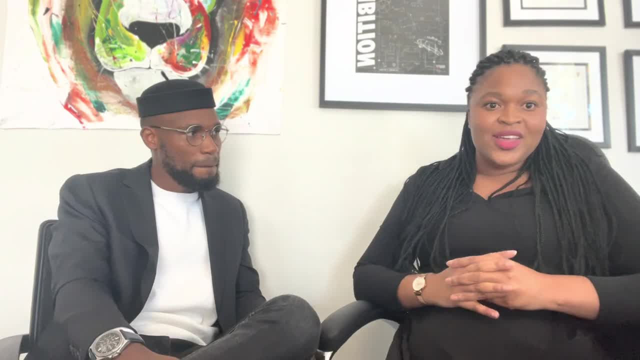 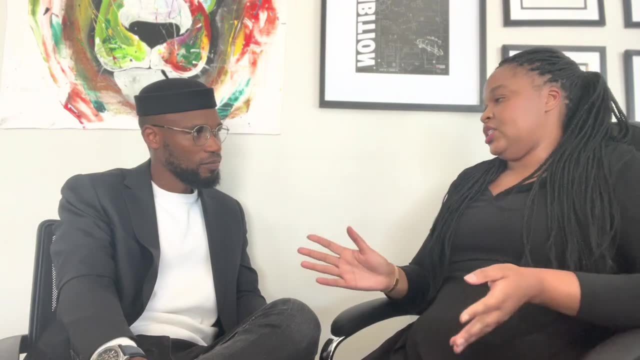 influence now is, I think it's recognized. Wow, Wow, That's really nice. So what's your intake in terms of tech in ACA? When we say tech in South Africa, what comes to your mind, What's your opinion about it? 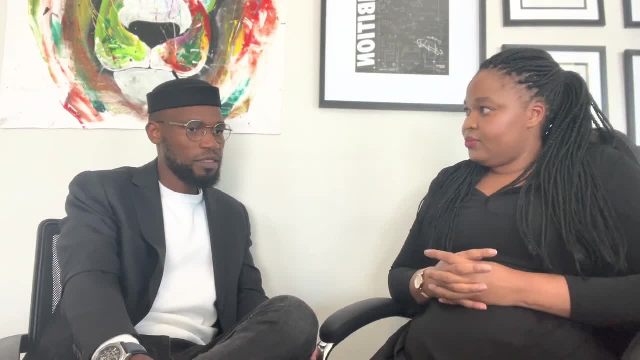 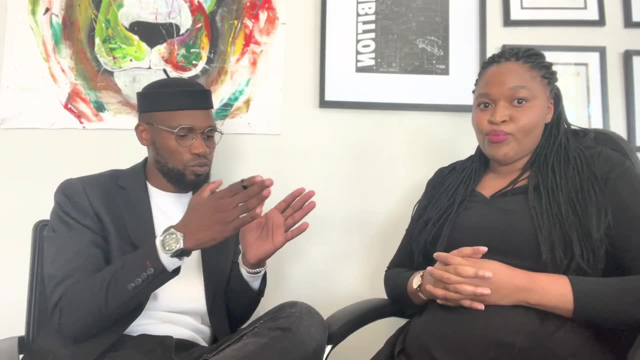 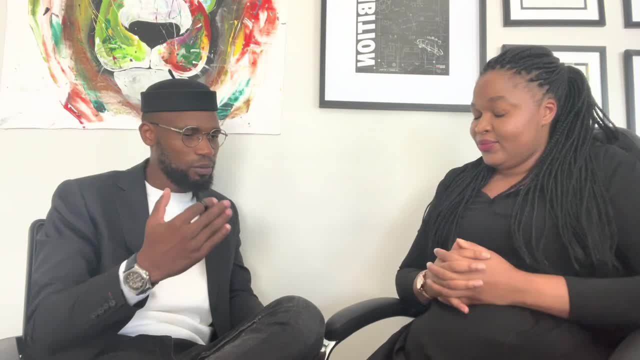 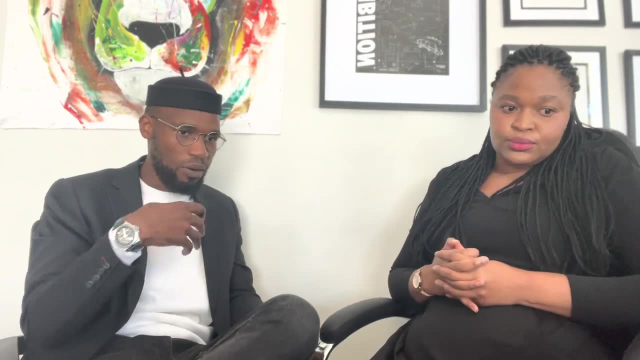 gives you five days to make a decision. if you had a system that gives you this real time, reporting real time- you are now able to make decisions real time. It automates the time it takes for you to grow And because of that, I feel like our company has been. 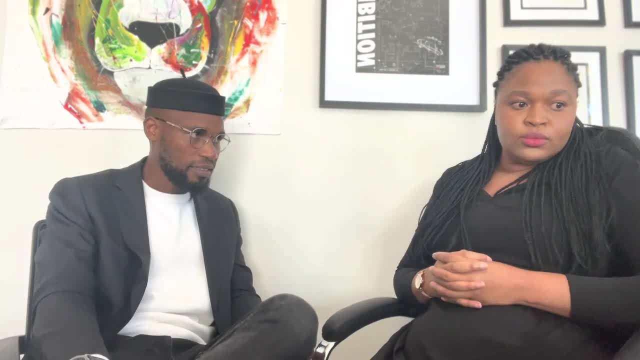 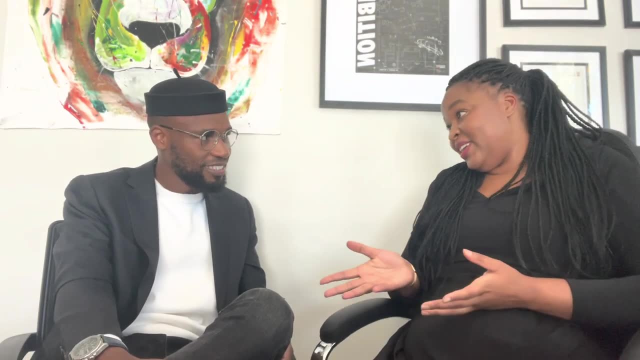 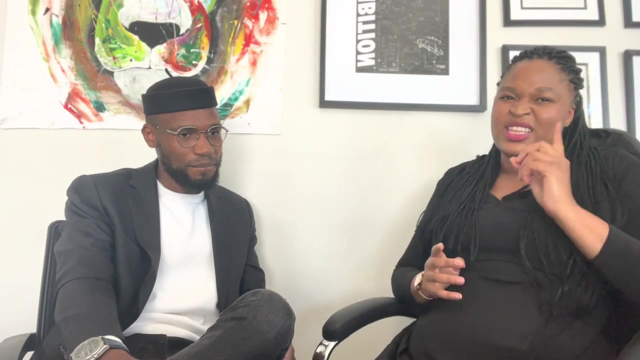 able to grow so fast because we are able to interpret insights. If you could, just like- I just want to add this thing, like: if you could, because you are feminine also- if you could pass one talent to your children, what would it be? Just that. 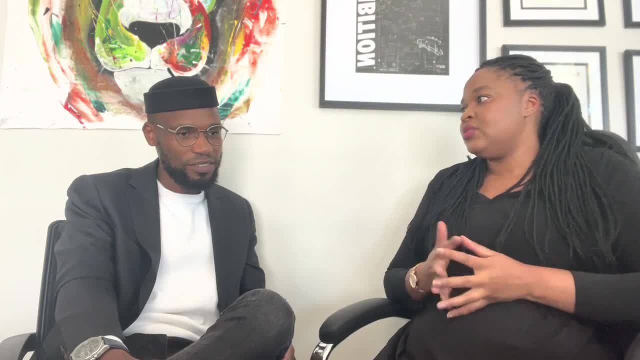 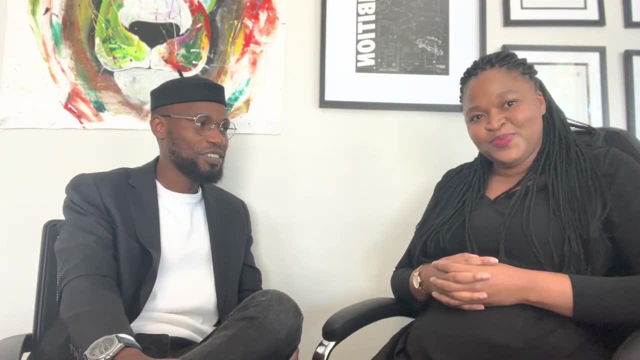 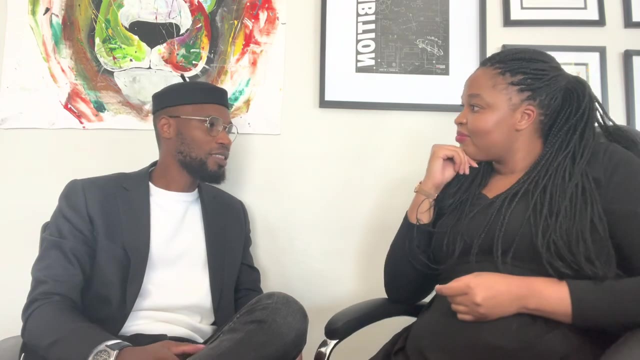 one talent to your children. you like want to pass this to my vision: vision, vision. man. money follows solution and solution come from vision. i have vision. you know what i've said with some ceos and they try to judge me. no vision, and i'm telling you the truth. i want them to see it. no vision, it's very hard to have. 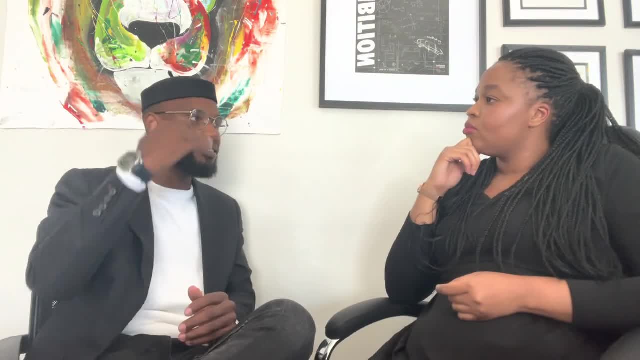 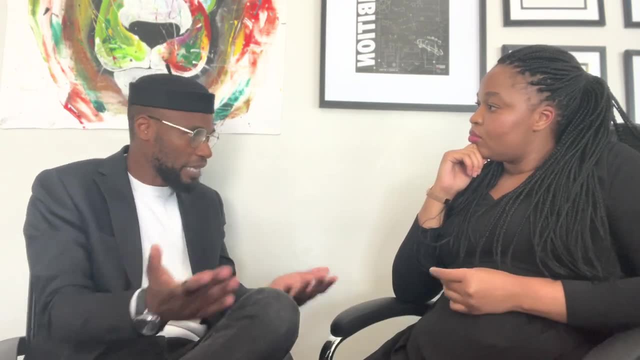 a person judging you and they don't have a vision because they don't understand it. everything i've said happened. everything i'm saying happens. if i'm saying we're going to uae, that's what i'm saying, but a person without vision don't hear it. if i had to pass that to my kid, i would say: have a vision. 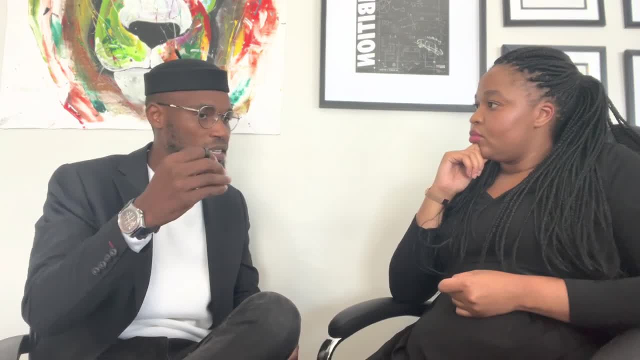 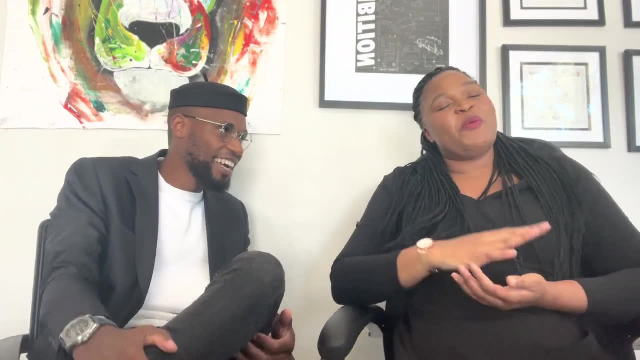 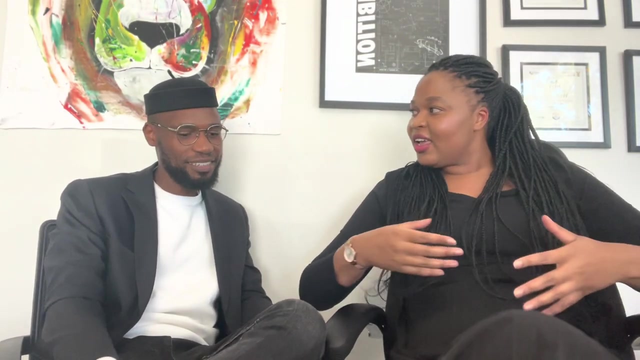 it doesn't matter whether they either hear you or not, because when you have a vision over time it makes sense. does this make sense now? wow, you just heard it from from mr banks himself. i mean, mr banks, multi-millionaire, you know, banking, the song that you. 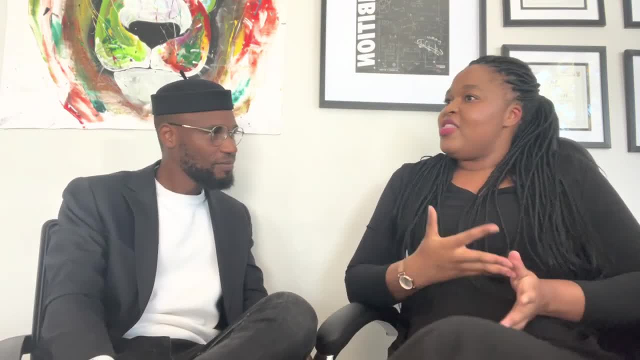 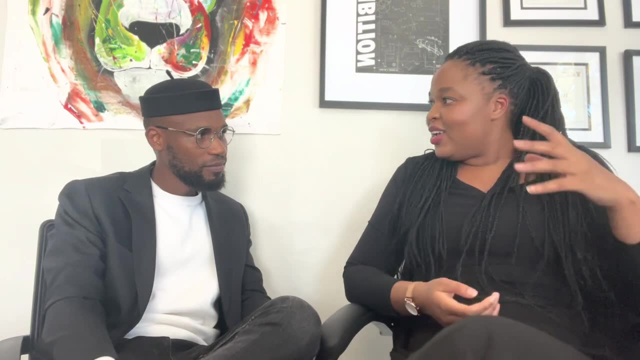 love. you know everything is about the moolah. so now that you're touching on the moolah side, what's that one thing that, after you've got your best deal, anyway, like you know what i'm buying myself, you know you can have vision, you can, but you have that one thing that you like: i won't move if i. 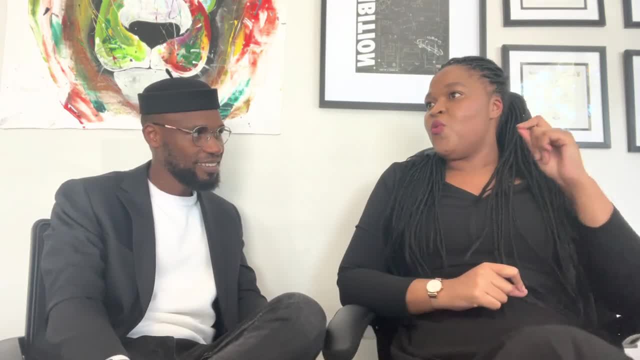 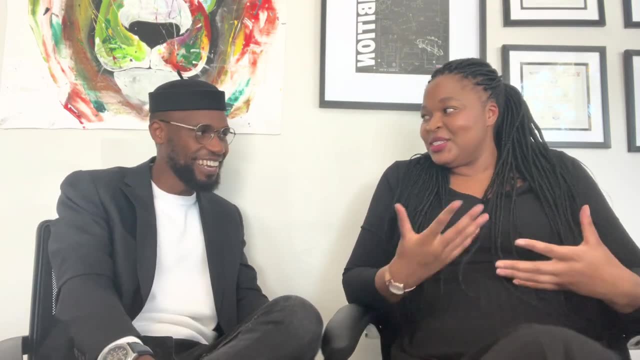 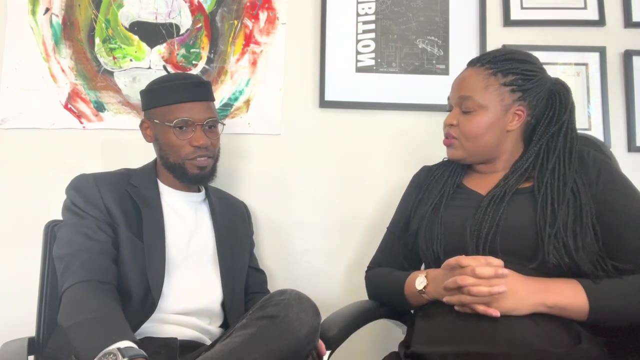 could get this one thing, this moolah, what's that one thing that you bought? and you were like: i bought a watch, but in a proper watch. you don't want to ask, yeah, i don't know, but you've got a watch. i gave it to my father now because it was not the biggest thing for me now. now, remember that time it. 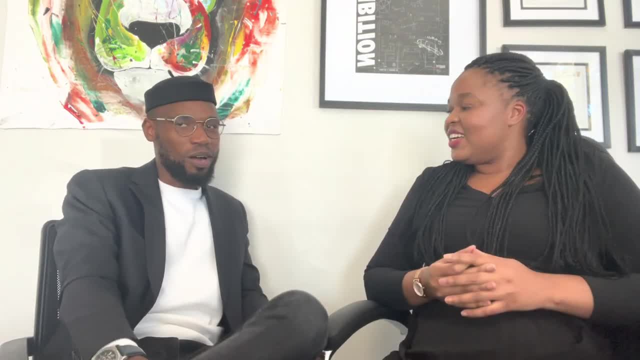 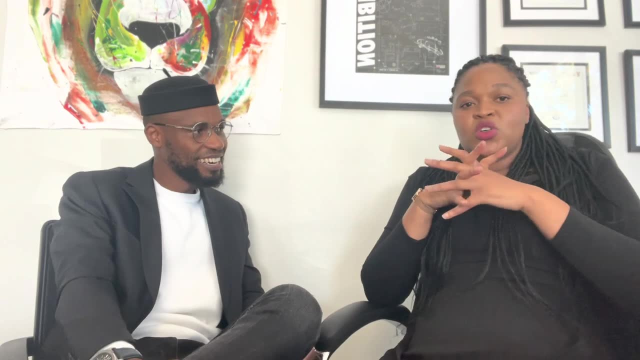 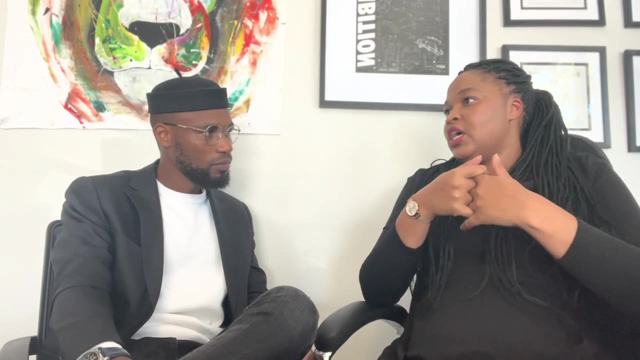 was: yes, yes, it meant something. yeah, i watched for like 40 000- you think yeah levels to this, you know. and also, um, also, i wanted us to talk about how the data science like in the company that you worked for- right, it's not like being a data scientist. do you get peanuts, you? you? 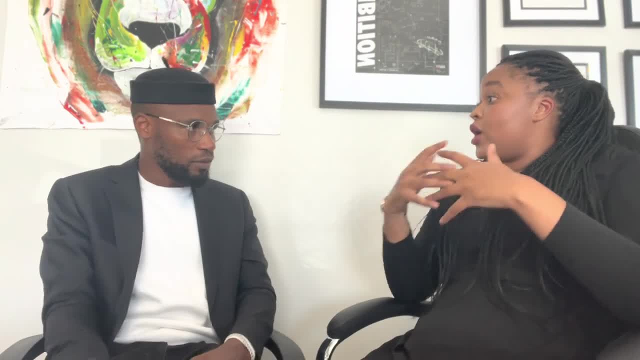 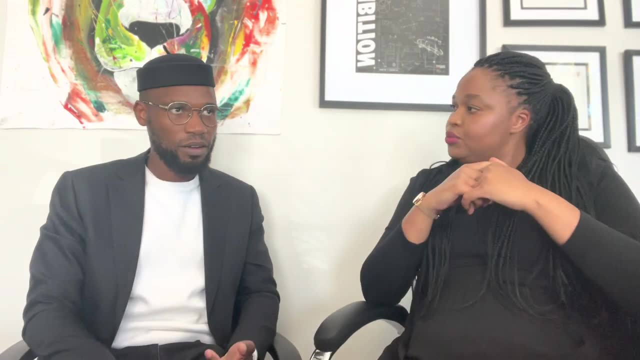 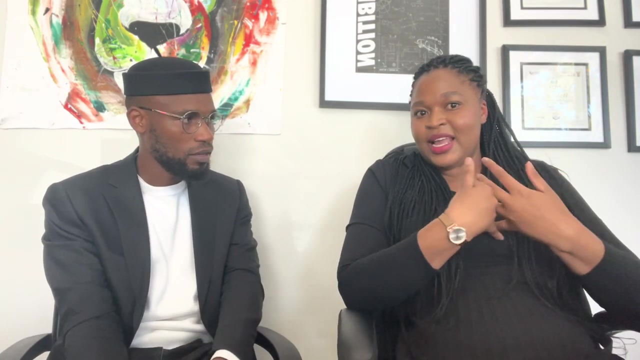 can make a living. you mean us here or where i was working. way, we're working. yeah, um. so i worked for mossman pick and pay, um, and auto zone, autozone. when i left us, i mean 45 thousand. see you guys, amazing, there's money in tech. there is money and there's money in tech. it's just that, for now it's. 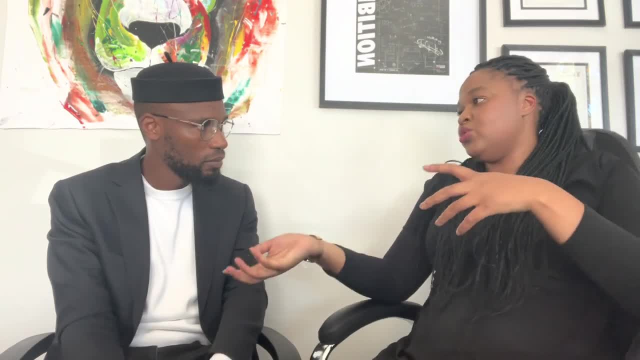 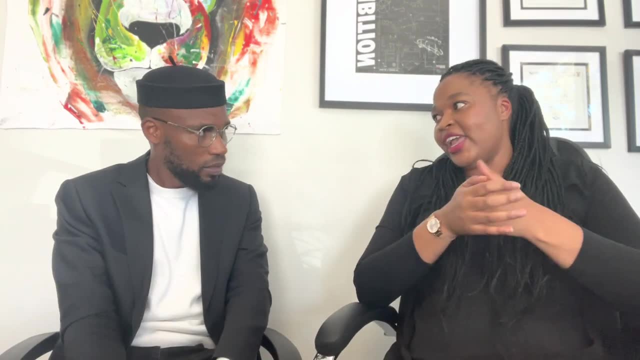 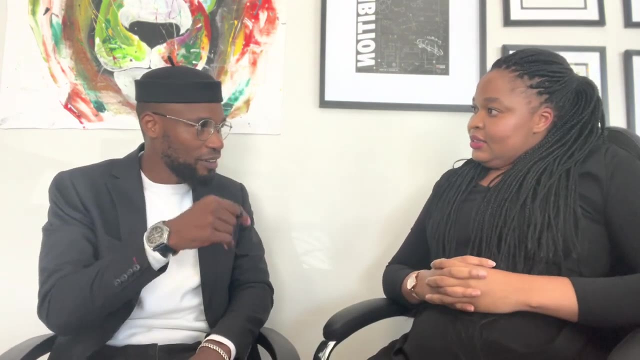 so funny how, when you read the news- um remember, i told you no on that- like connecting to other people, mmhm- and then the amount of money that they are coining and you compare it to the site you get. but you know what, like i started my first job, i was in 3.5, the first one that i'm saying i was 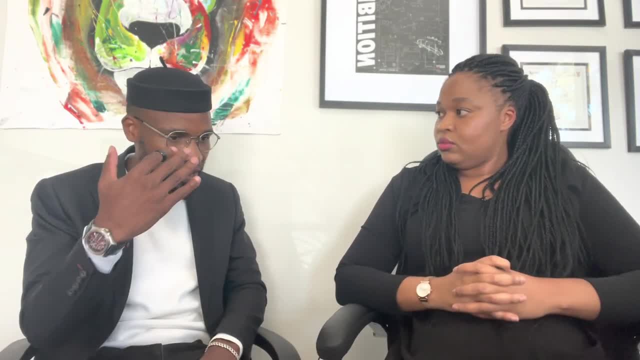 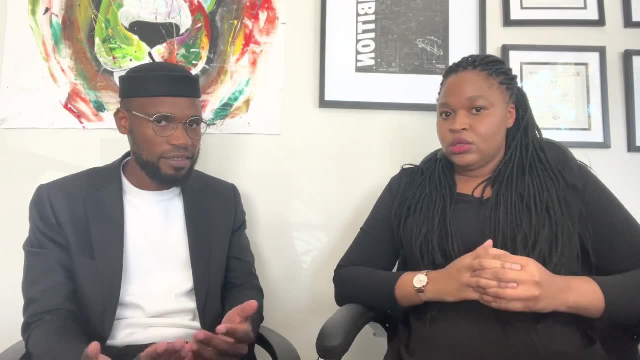 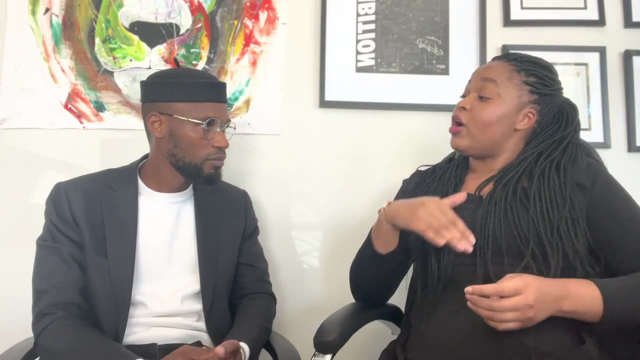 consulting, 3.5 it grew like. but from 3.5 you can make 45 000 and it takes show five years in. i was five years in incorporating, so already two years i was already doing. well, i had 2049 property and a car- oh, that's, that's so great. so, oh, you started, or at your first data, yes, but when i moved to when i was about to move, so i started working 2013, 2014. i had car and property, so it doesn't matter where you start with that. with 1000, you're gonna grow, you know. so what are you doing differently, uh, to what the normal corporate is, because i feel like you've been in corporate. 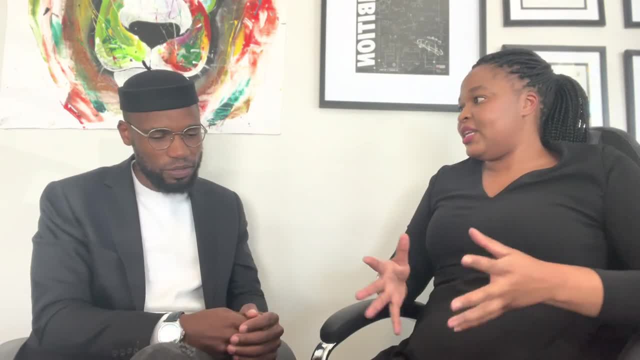 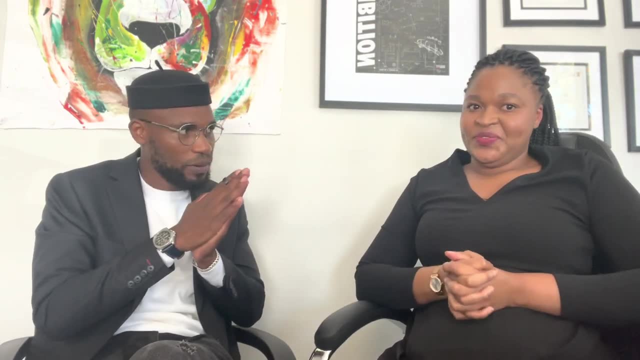 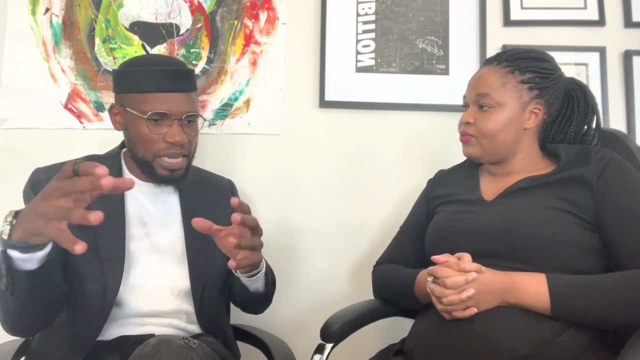 yeah. so you know the challenges, you know how hard it is, i know, but what are you doing differently now? okay, first thing for sure, corporate. one thing i can tell you: in corporate right, it's like it's a dog eat dog world. it's like i have to milk whatever and grow. 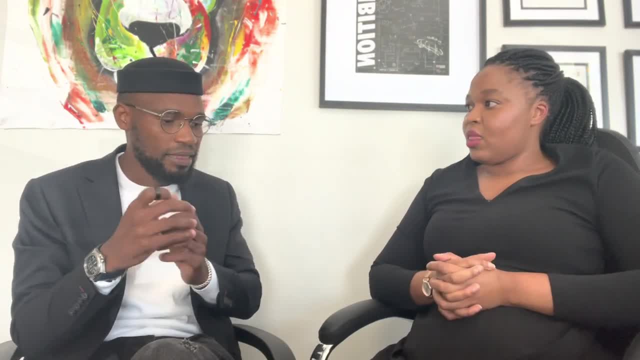 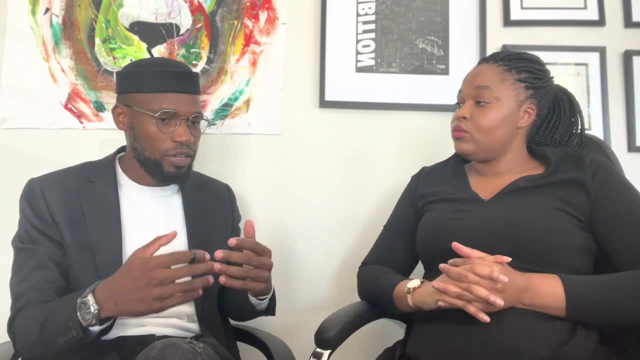 i don't believe in that and i i feel like that is based on selfishness. there's a lot of selfish people in corporate. they can send you out. you don't know who's who, so when you're talking you don't know what this person can say to you. there's a lot of hierarchy. 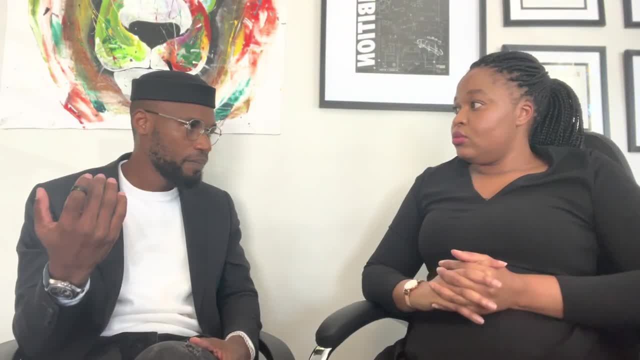 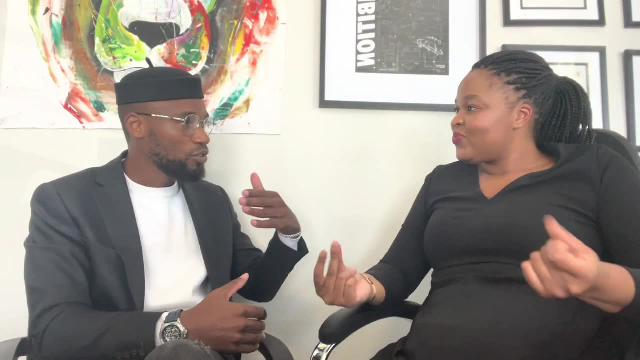 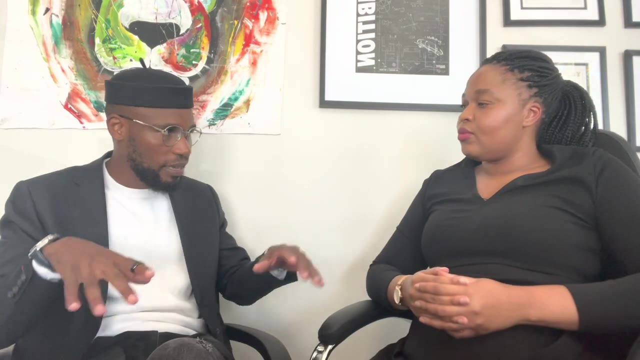 that can get you in trouble. you just find an email out of the blue: um. one thing we're doing right here is we are about energy connection. i connect with you, trust me. i hear you, and everyone here connects with each other. so there isn't hierarchy in our level. everyone is the same, and also energy doesn't. 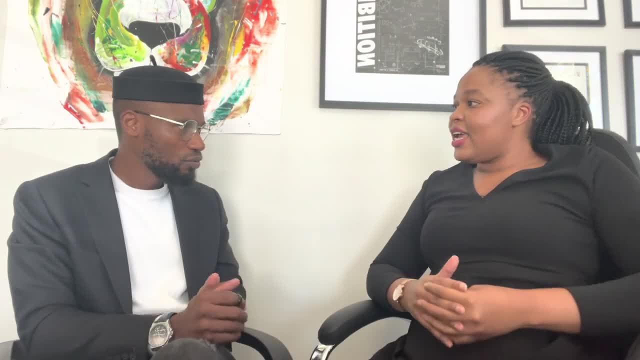 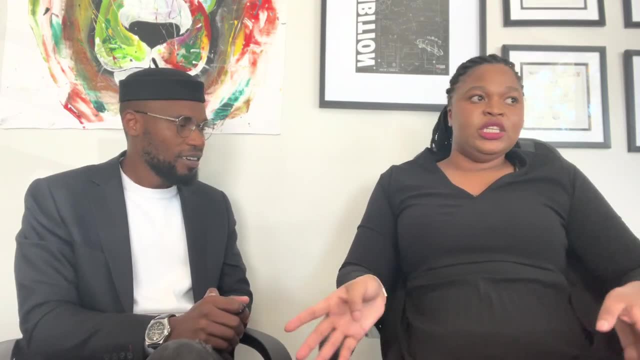 lie. i strongly believe. yes, energy tells you yes, and energy also tells you who to keep around your. yes, energy doesn't just leave you alone, just keep around your corner. energy doesn't just leave you alone. it's who you are, and if something is not giving you energy, you're not gonna do well and you can. 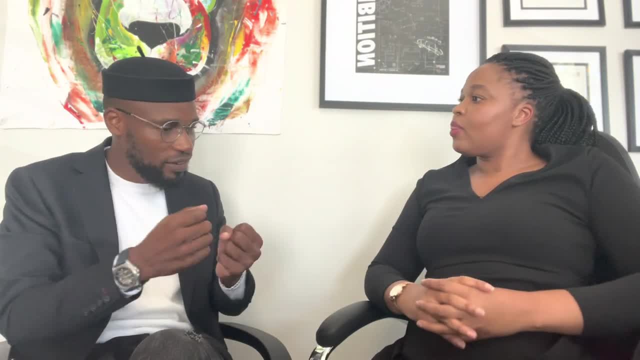 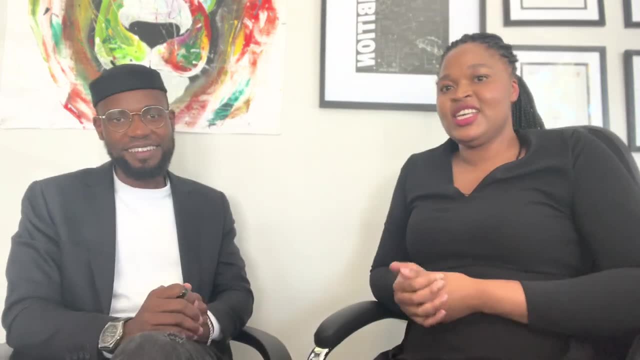 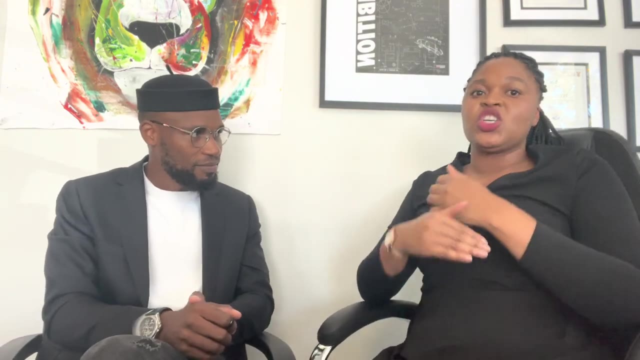 create without it. so that's why we're growing so far: because everything is being multiplied. everyone is multiplying themselves. because their energies are good. man, the energies are good. oh wow, thank you. i i feel even the energy right now. guys, i won't lie to you, it's good. 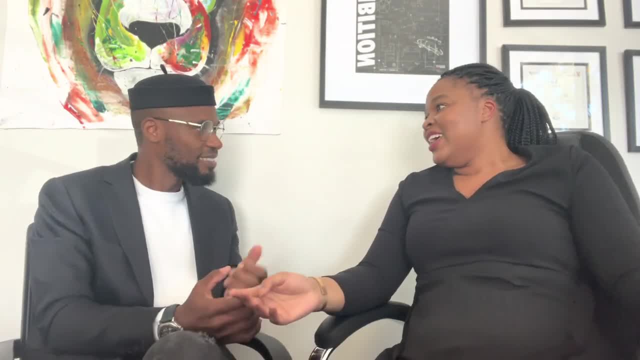 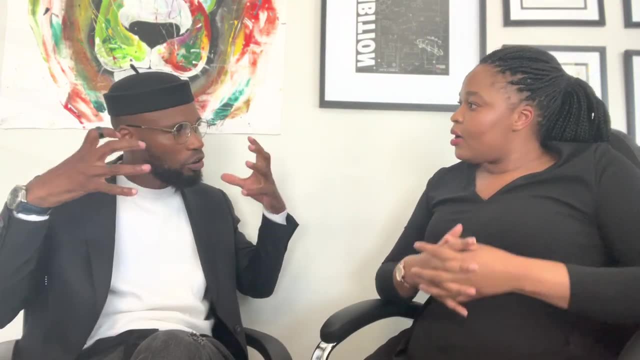 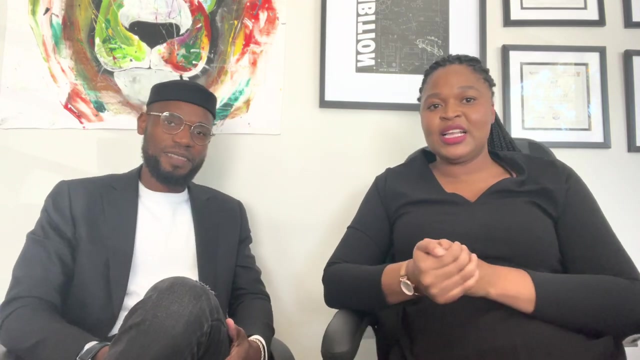 like i just got in and it's like i knew you from. it allows you to start creating, because now you are yourself and you want to like release all of that knowledge you had. you see what i mean? that's the whole point exactly. thank you so much. 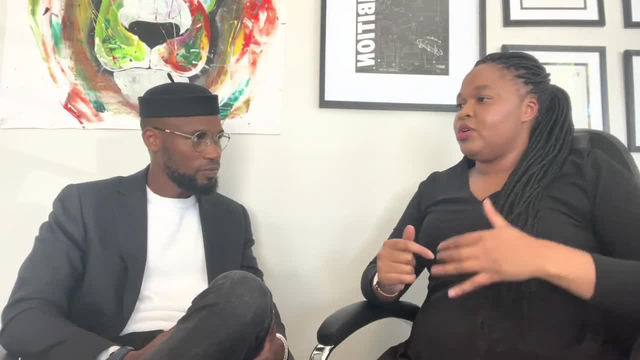 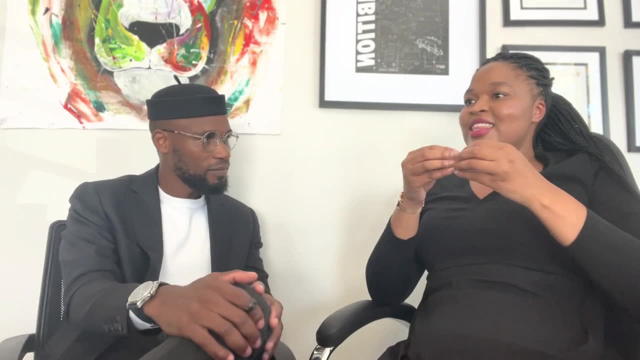 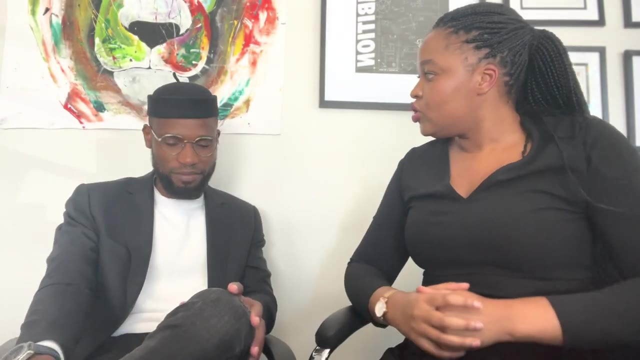 i want to talk about tech in the family because i feel like the reason these things are so slept on is it's because tech like it has this thing that you have to be stressed. hey, reporting lines from: yes, you know, do you get what i'm saying? so it doesn't have to come out professional. yes, and.